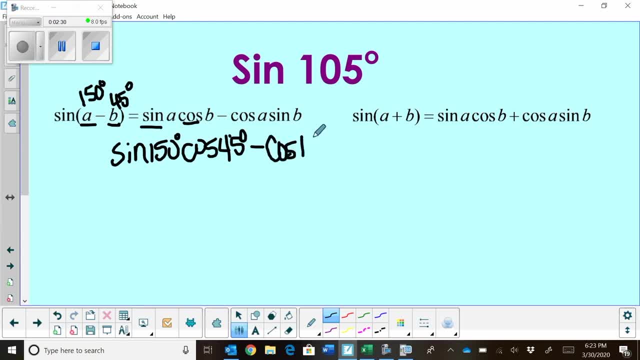 The cosine of A and A is 150, over the sine of B, and we know that B is 45 degrees. So that's how we would expand the difference formula: using values off the unit circle. So, and then we can just evaluate that, and we're going to do those in a minute. 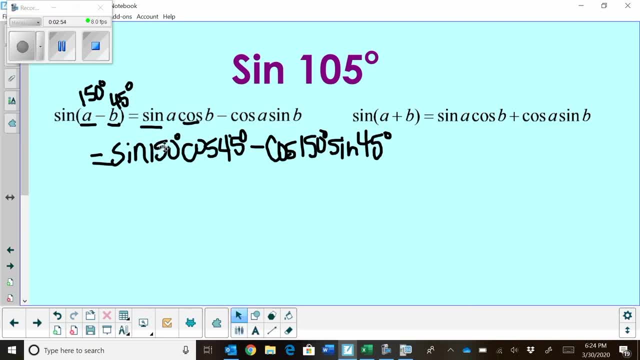 Okay now the sum formula is very similar to that. Let me grab all this and slide it over. It's sine A, cosine B plus cosine A sine B, So everything is the same except for literally the sine. 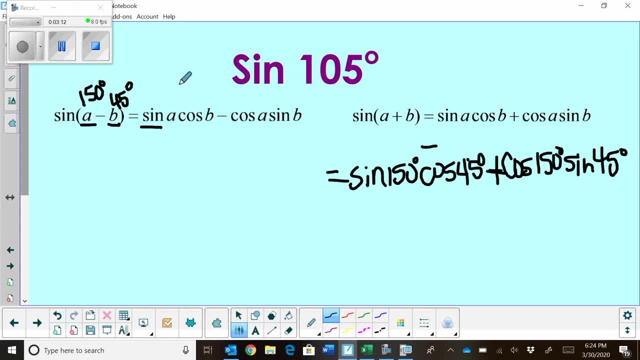 So this is going to be a positive, And how I always teach it is sine's formula is sine cosine, cosine sine, Same sine, And that last sine is S-I-G-N. the fact that we're subtracting. 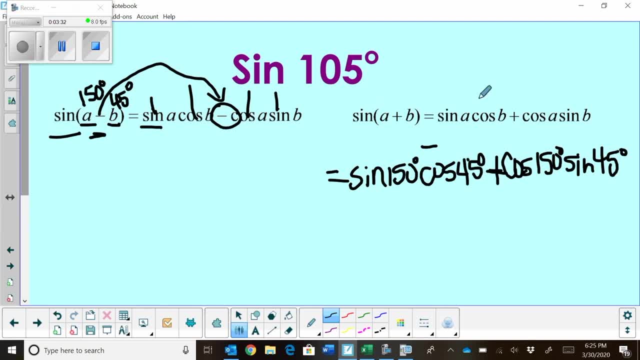 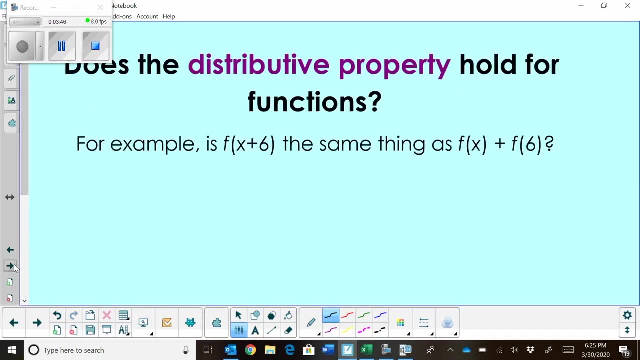 Therefore this is subtracting And the same with the sum formula: Sine cosine, cosine sine, same sine. So that's how you can remember the sine formula. Okay, Now, this one's kind of tricky because we need to talk briefly about the distributive process. 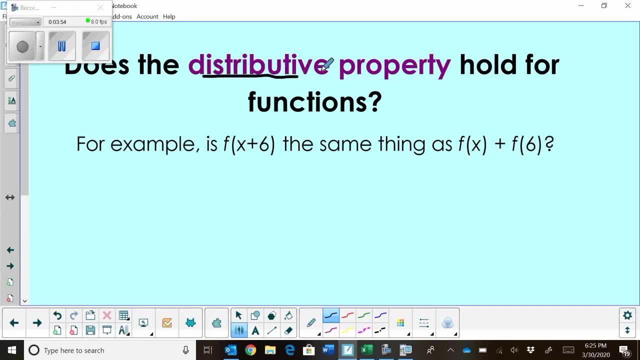 So let's talk about the distributive property. So does the distributive property hold true for functions? So if we have F of X plus 6, is that the same thing as F of X plus F of 6? Hmm. 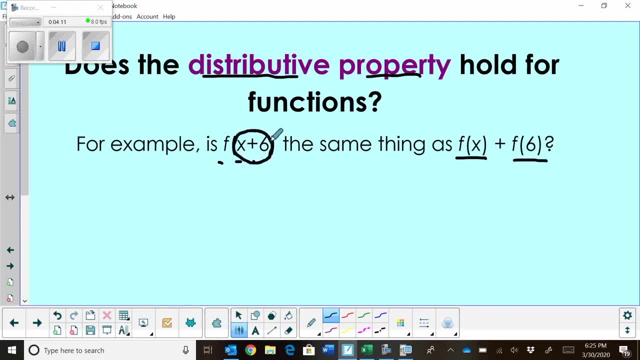 So if I take a value of X and I add 6 to it, am I going to get the same output as if I evaluate F of X, whatever X is, And then I add the value of F of X And I hope you're saying no, that is not true. 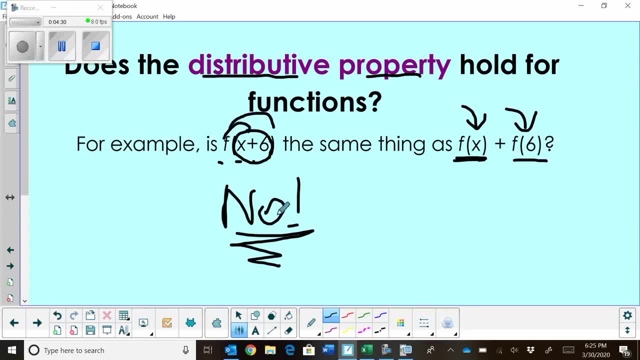 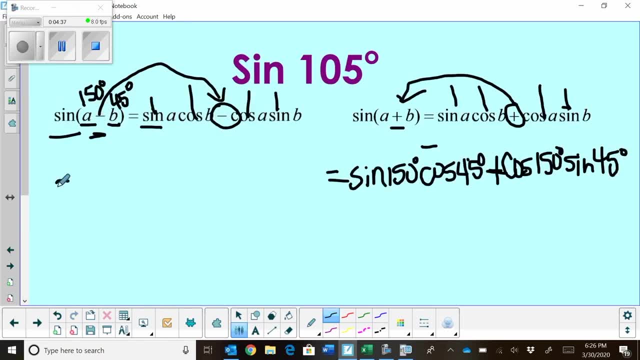 So the distributive property, or if we distributed that in, does not work. That's why, on this one, the sine of A minus the sine of B is not sine A minus sine B. That would be applying the distributive property to this sine formula. 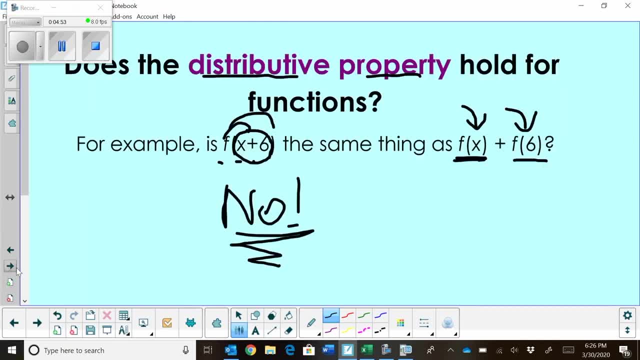 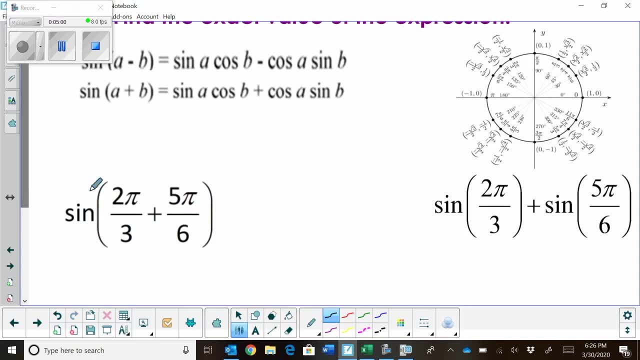 And this is not true. So, when it comes to functions, that's not true, Okay, And we can show you with an example. So here's sine of 2 pi thirds plus 5 pi sixths. We're going to evaluate it using the sum formula. 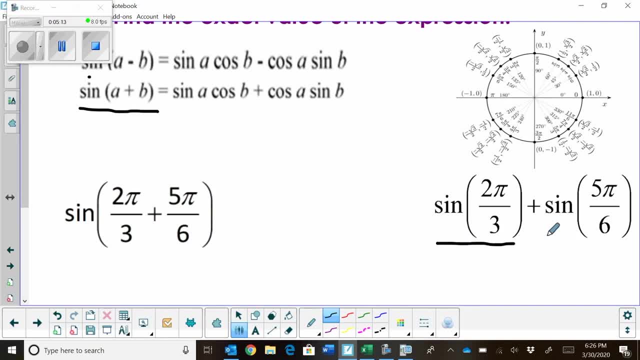 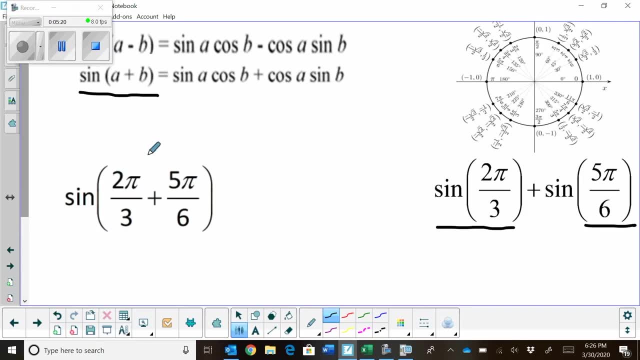 Then we're going to look at the sine of 2 pi thirds and the sine of 5 pi sixths and see what that is, And we're going to compare them to see if it is true. So let's evaluate this using our sum formula. 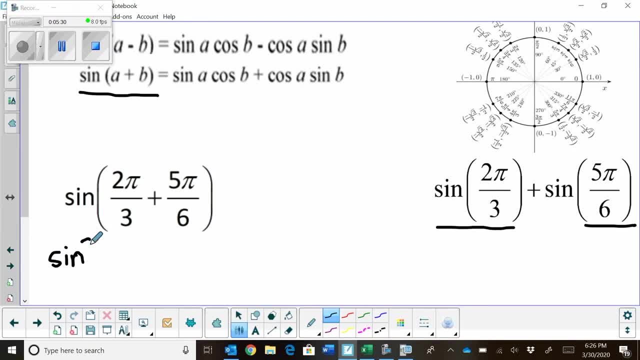 So I'm going to expand this with sine of 2 pi thirds times the cosine of 5 pi sixths, And I'm going to add to that the cosine right of the first one first angle, which is 2 pi thirds. 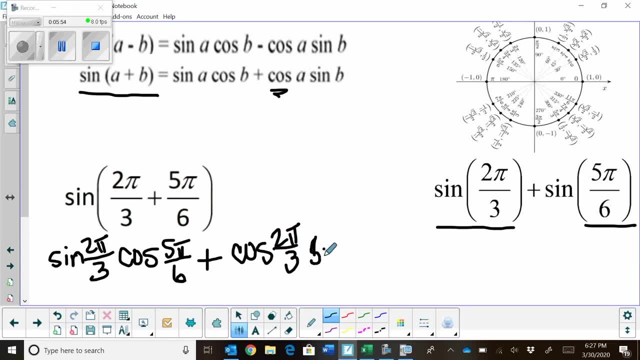 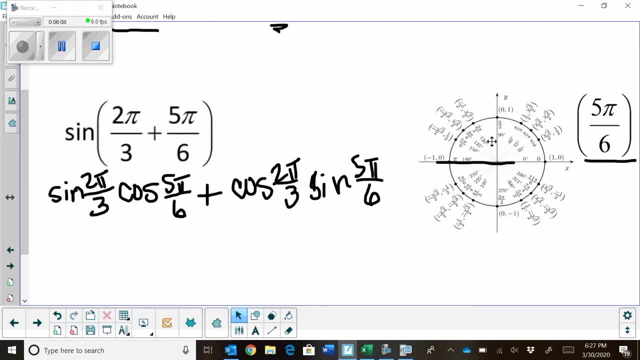 Times, the sine whoops, the sine of 5 pi sixths, And let's evaluate that off the unit circle. So if you need to, you can grab your unit circle. We can look at this, Okay: Sine of 2 pi thirds. 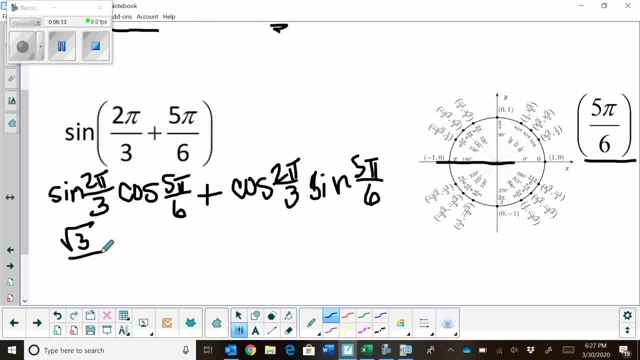 That is a root 3 over 2.. Times cosine of 5 pi sixths. That's right here And that is negative root 3 over 2.. We're going to add to that the cosine of 2 pi thirds, which is negative 1 half. 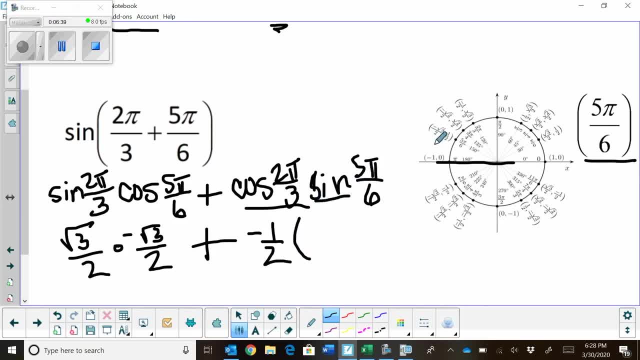 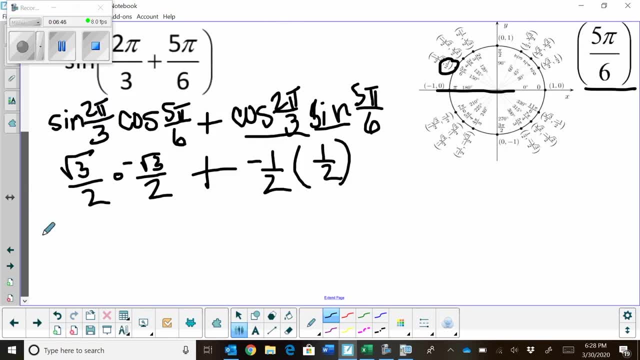 And we're going to multiply that times the sine of 5 pi sixths. Well, the sine of 5 pi sixths is positive 1 half. So let's multiply all that together, That's going to give me negative root 9.. 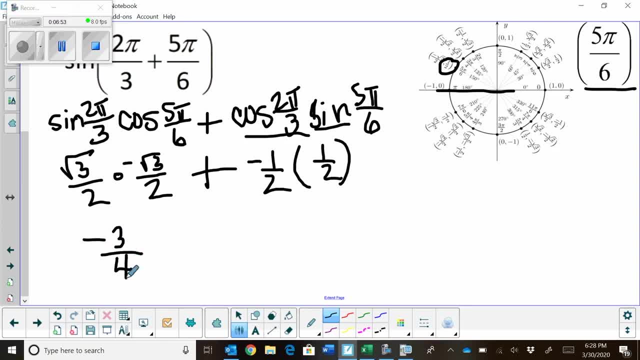 Which is 3 over 4.. And I'm going to add to it actually a negative 1 fourth. So that's going to be plus a negative 1 fourth. Well, that ends up being negative 4 fourths or negative 1.. 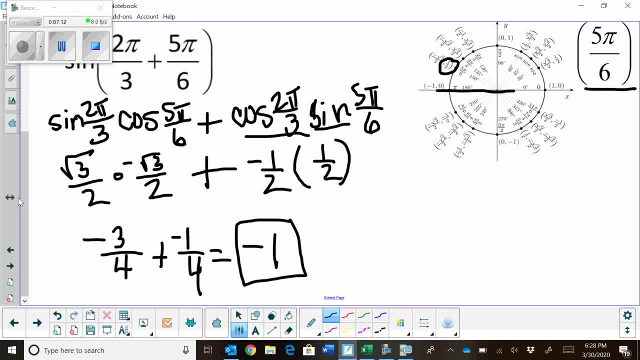 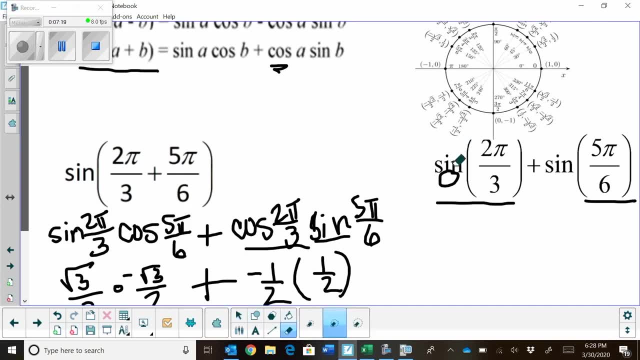 So there's the actual answer. Well, do we get the same thing if we evaluate as if we've distributed that in? Well, let's do that, Let's try it, Okay. So what's the sine of 2 pi thirds? 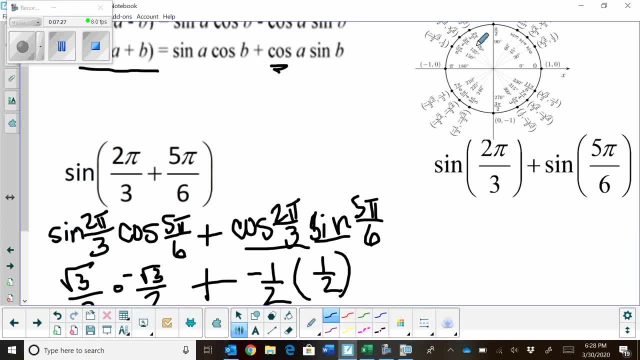 Well, we actually used it over here. Okay, The sine of 2 pi thirds would be- and I'll try to slide this down so you can see it- The sine is root 3 over 2, which hopefully by now you have that memorized anyway. 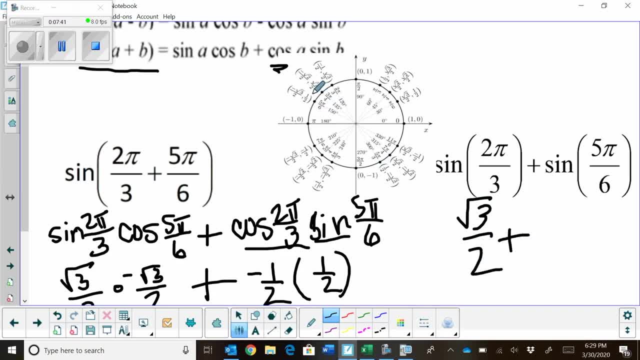 We're going to add to it the sine of 5 pi sixths. Well, 5 pi sixths is 1 half, So if we add those together we just get root 3.. Plus, Plus a positive 1, all over 2.. 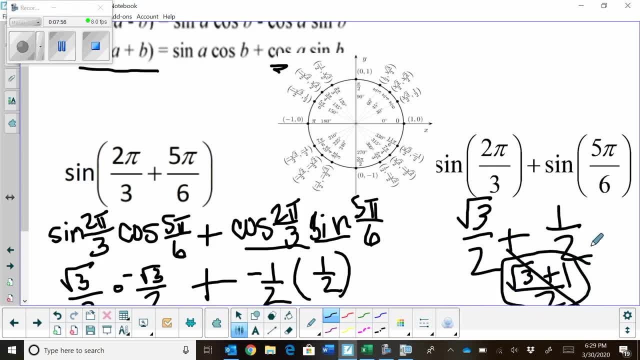 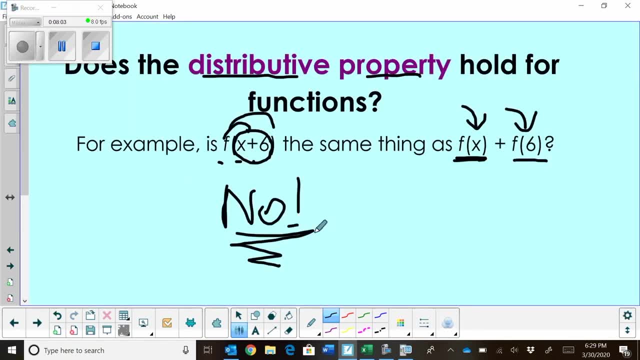 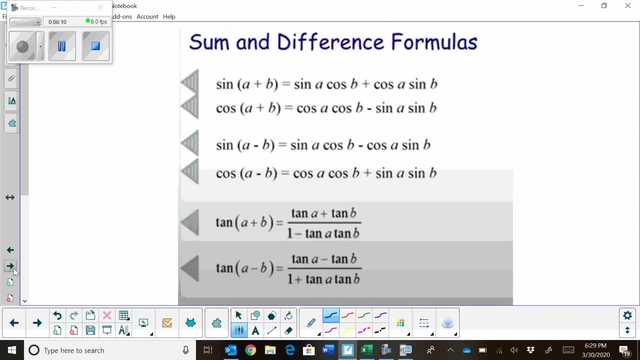 And that value is not 1.. So, guess what? These are not equal. Therefore, you cannot distribute it. It supports the fact that this is a no, They are not the same thing. Okay, So what are our sum and difference formulas? we're going to work with in this lesson? 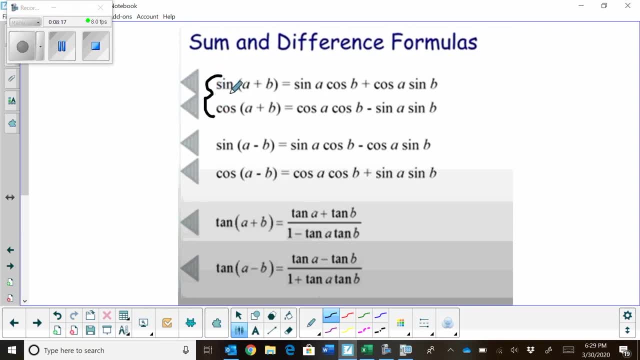 We're going to work with the sum of cosine and the sum- Sorry, Cosine- and the sum of sine. We've already looked at the sum of sine And it's sine, cosine, cosine, sine, same sine, But cosine of the sum is a little bit different. 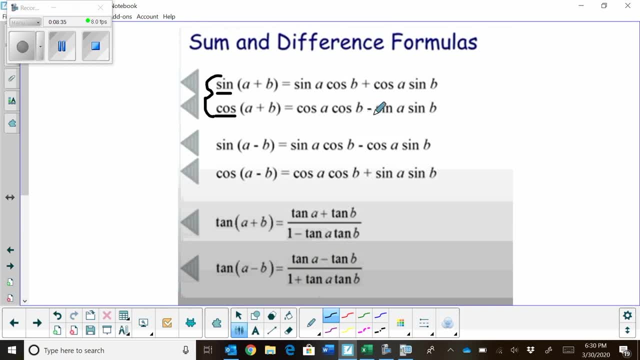 It's cosine cosine minus sine sine. So it's cosine cosine sine sine opposite sines, And the same thing is going to work for the difference formula Sine is sine A, cosine B, So sine cosine, cosine sine. same sine in the middle. 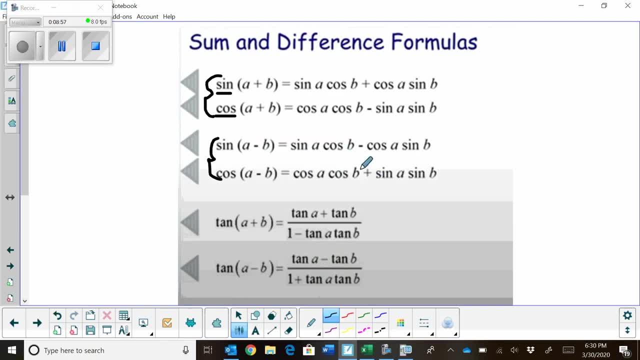 But cosine is cosine, cosine plus, So it's the opposite sine of sine sine. So you multiply the cosines together, multiply the sines together, and it's the opposite sine. And then tangent's got its own pattern. 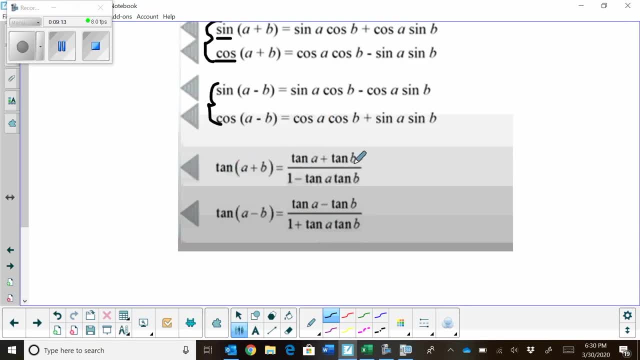 Tangent. you're going to take the tangent of A plus the tangent of B, So it almost looks like you do distribute it, But then you're going to divide it. You're going to divide it by 1, minus their product. 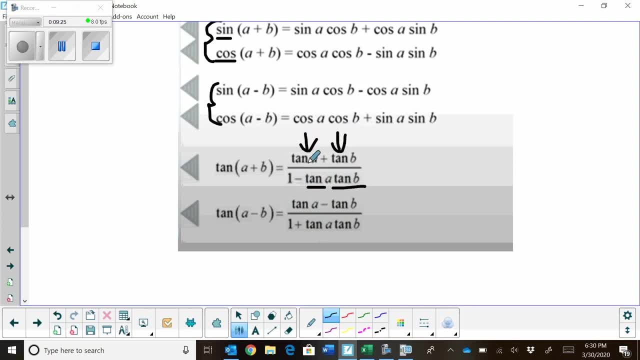 So, whatever you get up here, you're actually going to subtract that product from 1.. Okay, And then for tangent of the difference, it's tangent A minus tangent B. So notice the numerators are the same, But what do we notice about the denominators? 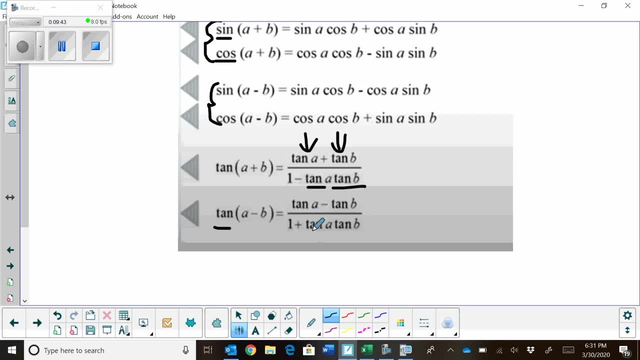 They're the opposite. So this will be tangent A times tangent B. So tangent is the same sign on top And the opposite sign on the bottom. You apply the operation to the tangent of A plus or minus on top, the tangent of B. 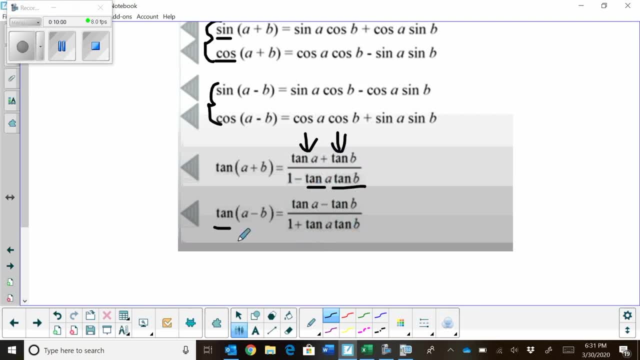 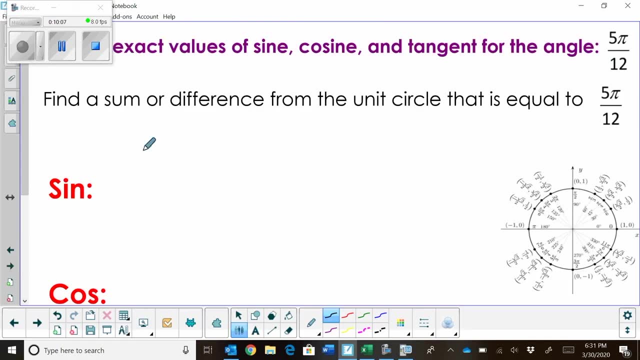 And then 1 minus or plus, the product of tangent of A times tangent of B. Okay, Keep those formulas handy because we're going to use those to evaluate now. So find the sum or the difference from the unit circle of the value 5 twelfths. 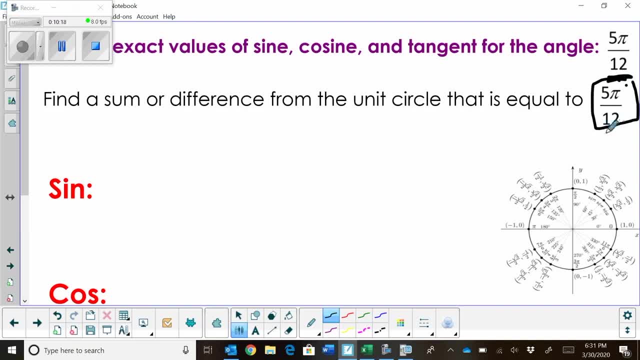 So we need to come up with two angles That are on the unit circle, that add or subtract to 5 pi twelfths, Because 5 pi twelfths is not on the unit circle, But we could take 5 pi twelfths and divide it into two parts. 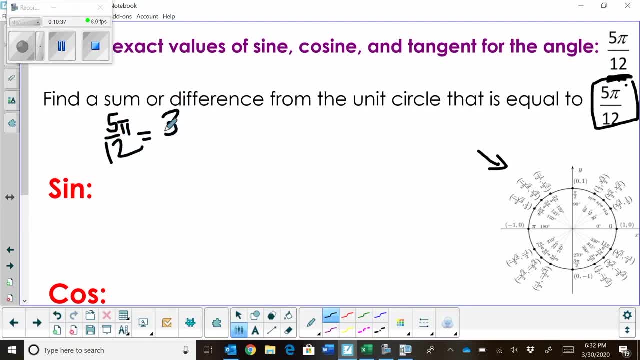 We can rewrite that as the sum of 3 pi twelfths and 2 pi twelfths, That's 5 pi twelfths. Okay, Now We don't recognize those because they're not reduced, So let's reduce those. 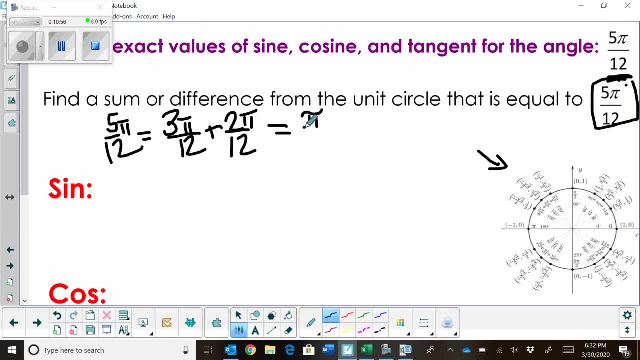 Okay, 3 pi twelfths is really pi fourths, And 2 pi twelfths is really pi sixths. So there is our sum of the two angles. So let's write this out. So we have the sine of pi sixths or pi fourths. 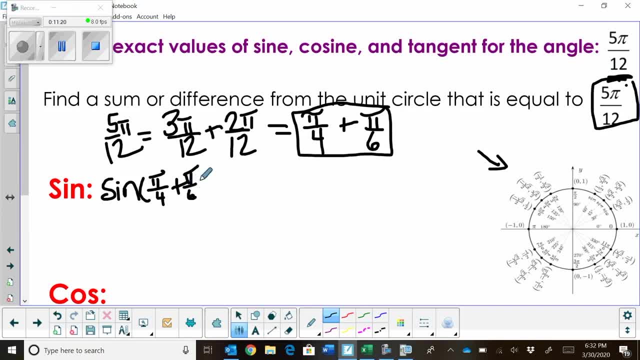 Plus pi sixths. Okay, So now I'm going to expand this using our formula. Now, sine is sine cosine, cosine sine, Same sine in the middle. So this is going to be sine of pi fourths times cosine of pi sixths. 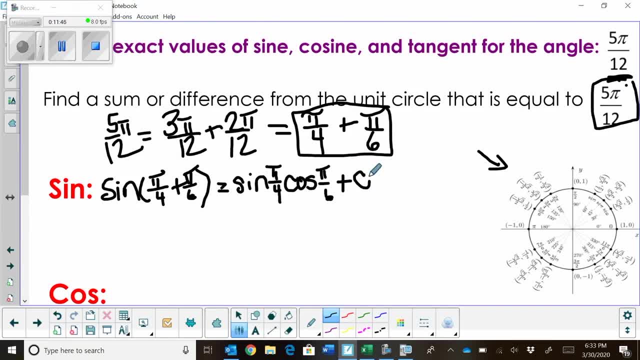 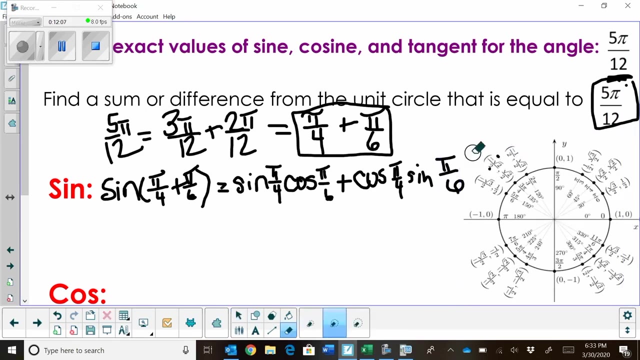 Plus Same sine in the middle Cosine. So sine of pi fourths times sine of pi sixths. Now let's use our unit circle, if you need it, to evaluate those values. So get comfortable again with the unit circle. 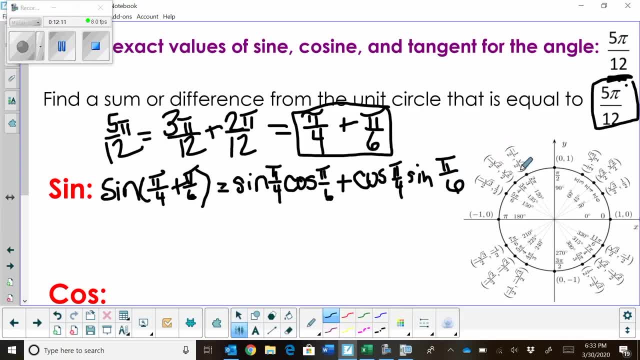 Remember, a while back I said, ah, it never really goes away. Okay, So here it is rearing its head. So sine of pi fourths is just root 2. Over 2.. Cosine of pi sixths is square root of 3.. 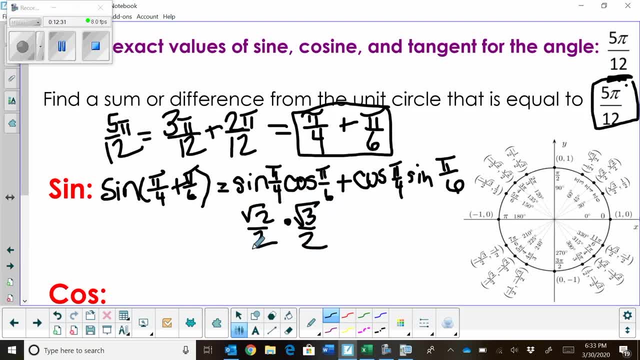 Over 2.. So the first portion of this is the product of those two values Plus. Well, the sine of pi fourths is the same as the cosine of pi fourths, which is just root 2 over 2.. And then the sine of pi sixths is a half. 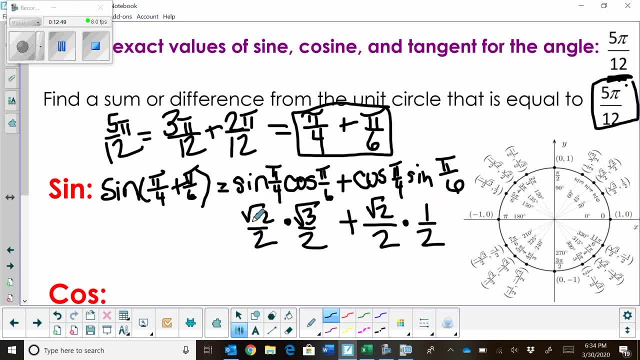 And we're going to find that And we're going to find that product. So what is that? Once we multiply and add, what do we get? We get a pi Or, I'm sorry, A root- 6 all over 2.. 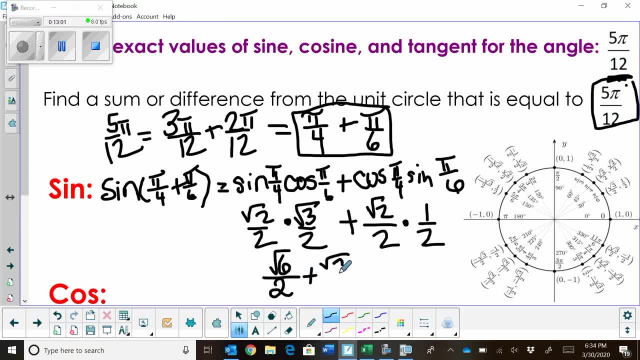 Plus a root 2 all over. oh, I'm sorry, My denominator is not 2.. My denominator is 4.. 2 times 2 is 4.. Sorry about that. And then root 2 over 4.. And then so our final answer is root 6 plus root 2 all over 4.. 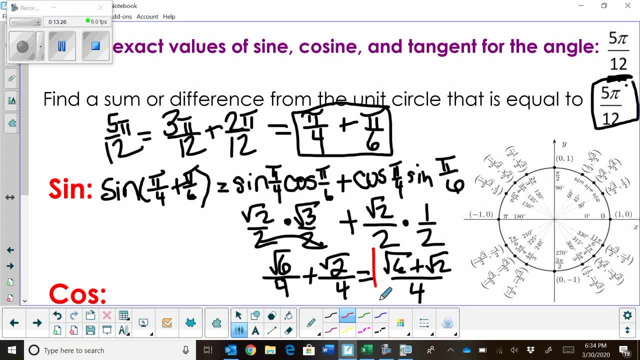 Now I want you to think. Can you simplify that? The answer is no. Root 6 does not add with root 2.. The radicals have to be the same in order to add those together And they're not divisible all by 2 because the 4 is not in a radical. 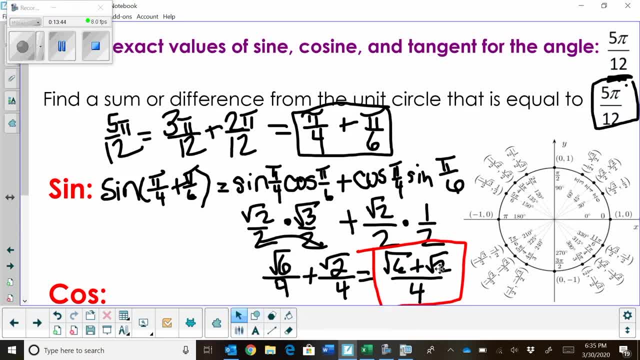 So you're done. It's just root 6 plus root 2. All over 4.. Okay, I'm going to move this answer over here, just in case we need to erase a little bit And make some more room for the next problem. 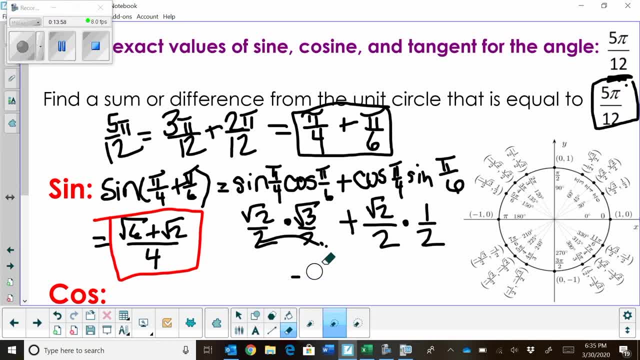 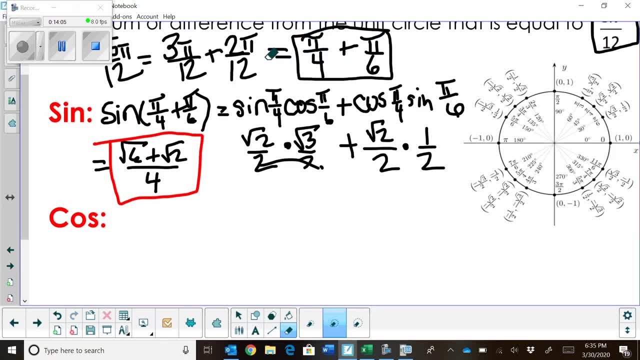 Oops, It's supposed to be an eraser. There we go. Now let's try the same thing with the cosine formula. So we're still going to find the cosine of 5, pi 12ths. We're just going to do that. 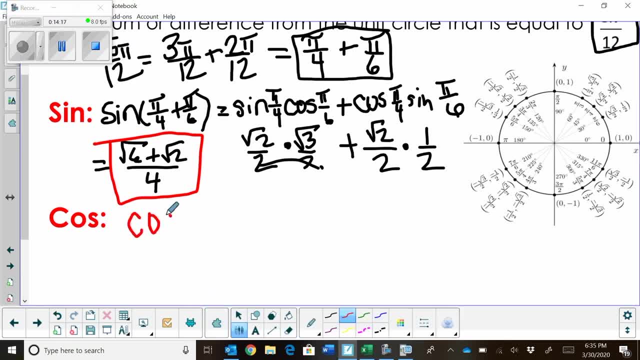 By rewriting it as the cosine. So let's go ahead and write it like that first. So what's the cosine of 5, pi 12ths? Well, we don't know that from the unit circle, So we're going to rewrite this as the sum of pi 4ths plus pi 6.. 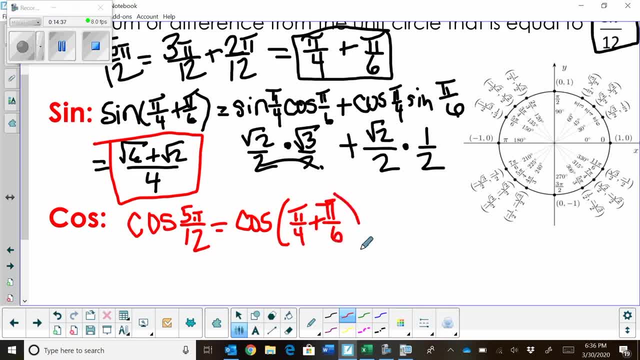 Because those two angles add to 5 pi 12ths. Now let's expand our cosine formula. Cosine works like this: Cosine, cosine, Sine, sine, Opposite sine in the middle. So we're going to write this as cosine of pi 4ths times cosine of pi 6.. 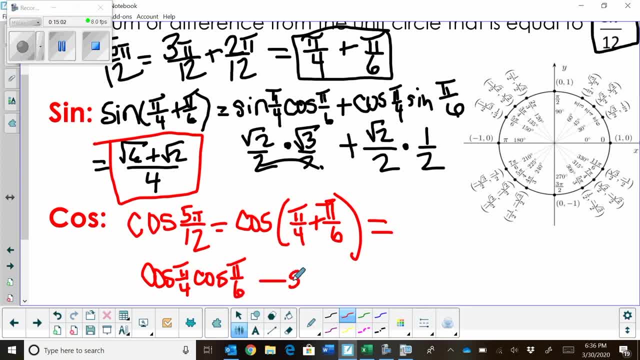 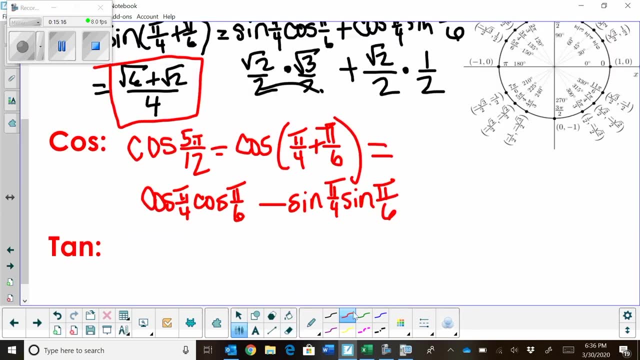 Opposite sine. So minus sine of pi 4ths times sine of pi 6.. Okay, And again you can use your unit circle if you need to. Hopefully again we're weaning ourselves off that. But cosine of pi 4ths is our root 2 over 2 times the quantity of cosine of pi 6.. 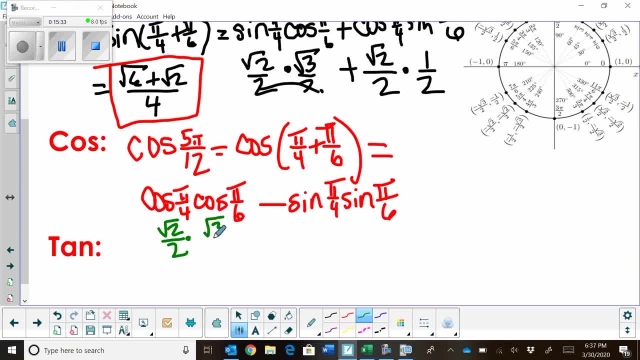 Well, that's just root 3 over 2, minus the quantity. sine of pi 4ths, That's root 2 over 2. And sine of pi 6. That's a half. So we end up with the quantity. 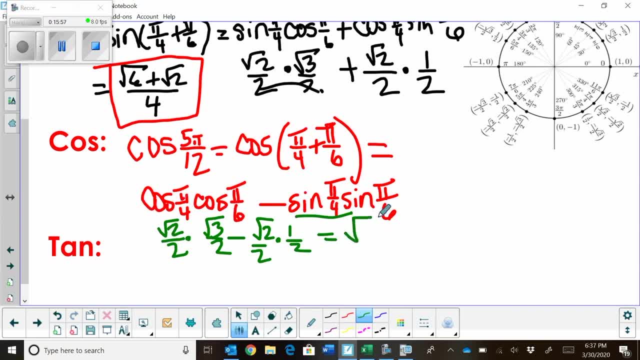 Well, the first term is going to be root 6 all over 2 times 2.. I won't do it this time. That's 4 minus root 2 all over 4.. So if we clean that up and just put those together, we're going to get a root 6 minus a root 2 all over the quantity 4.. 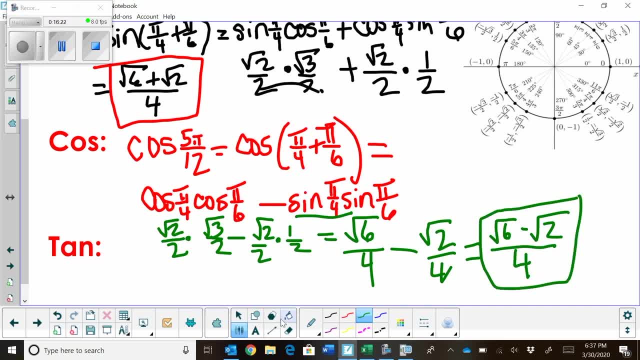 So, as we said earlier, we can't simplify that, But I want you to notice these two answers. They're very similar: One's addition and one's subtraction. It just ends up that way. There's always a little pattern to those. 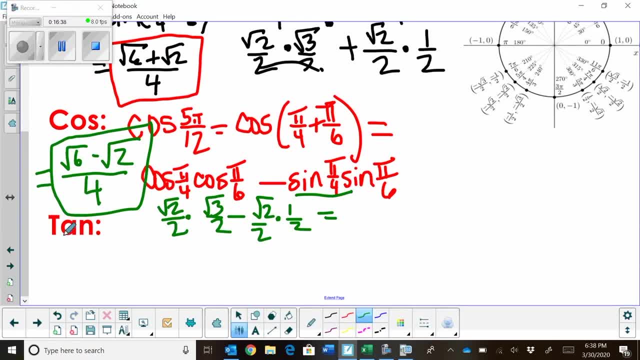 Okay, So now let's try the tangent. So we want to find the tangent of 5 pi 6.. I'm sorry, 5 pi 12ths, And we're going to rewrite it How, With the sum of the two angles. 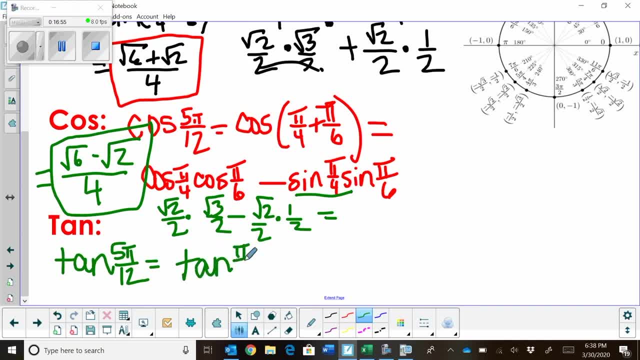 So tangent of pi 4ths plus pi 6.. Now our tangent formula is a fraction, So that makes it a whole lot trickier. Okay, So on top we're going to write it as tangent of pi 4ths plus tangent of pi 6.. 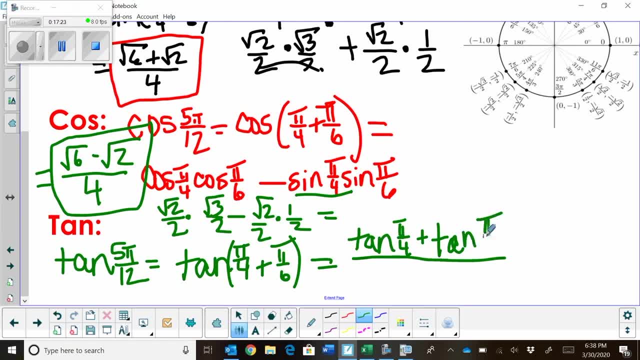 So it looks like we just distributed that on top And then on the bottom. it's always 1 and then the opposite sign, So 1 minus their product. So this is going to be still the tangent of pi 4ths times the tangent of pi 6.. 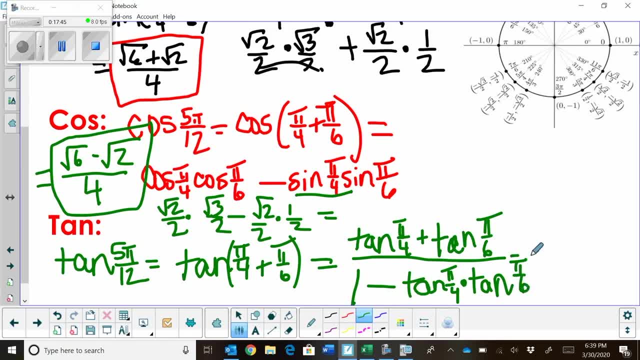 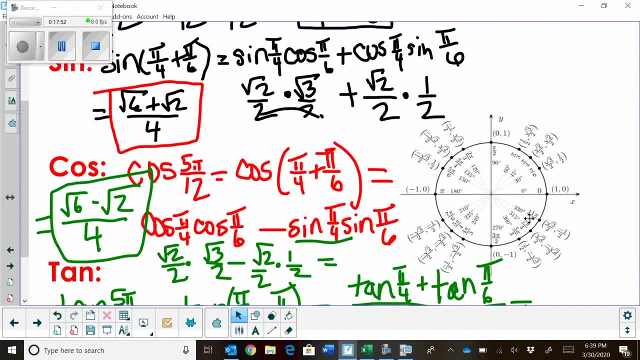 So let's see if we can figure this out. So on top, let's go back. What is the tangent of pi 4ths? So again, if you need your unit circle, just bring it down. Let's look at it. 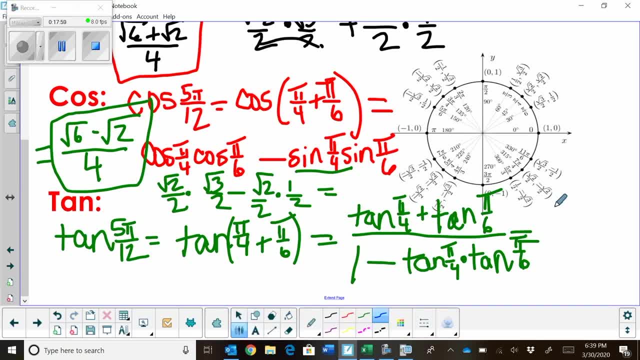 Tangent at pi 4ths. Hopefully you remember that- 1 plus what else is on top Tangent of pi 6? right here We know that's a root 3 over 3.. Okay, And then on the bottom we have 1 minus the product of those two. 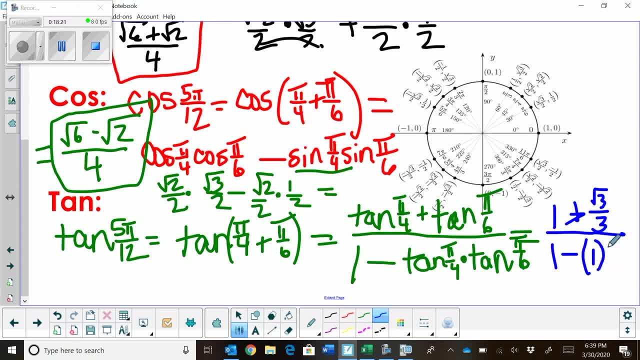 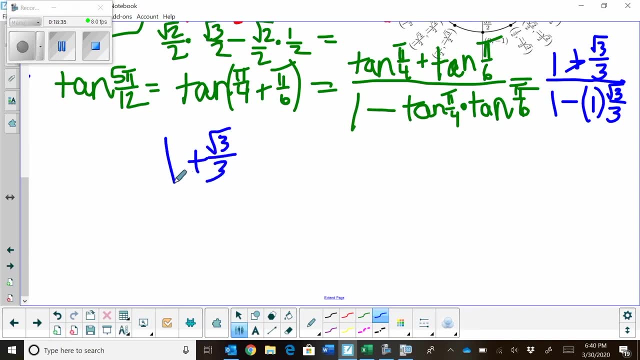 So the tangent of pi 4ths is 1 times root 3 over 3.. So let's just kind of clean this up a bit. So we have 1 plus root 3 over 3 all over 1 minus root 3 over 3.. 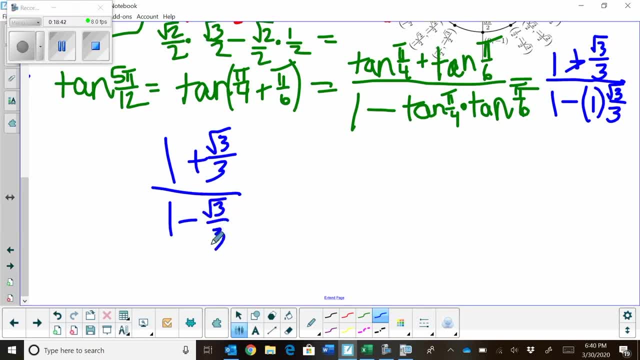 Okay, Now don't think that you can just, oh, I'm going to cancel my 1s out. No, no, no, no. This is one quantity and that is one quantity. They are totally different And you cannot, you can't cancel anything out here. 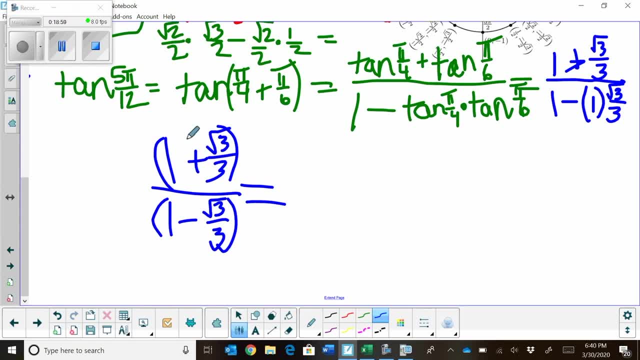 We can get common denominators and combine the top and bottom. So I'm going to now combine the top to 3 plus root 3 over 3.. Now hopefully everybody knows what I just did. I just multiplied 1 by 3 over 3 to get to rewrite that as 1 and then added the numerator. 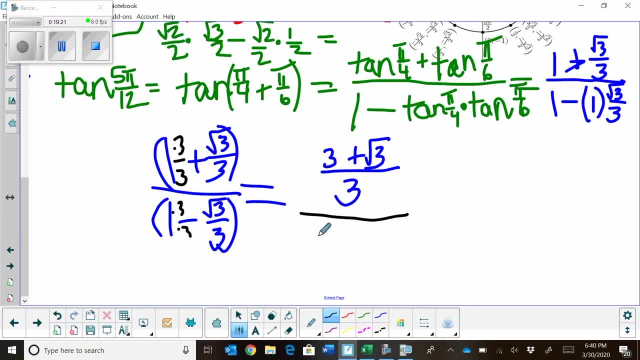 Then on bottom, I'm going to multiply this by 3 over 3.. That's going to be give me 3 minus root, 3 all over 3.. Now, hopefully by now you know some of the tricks of the trade. 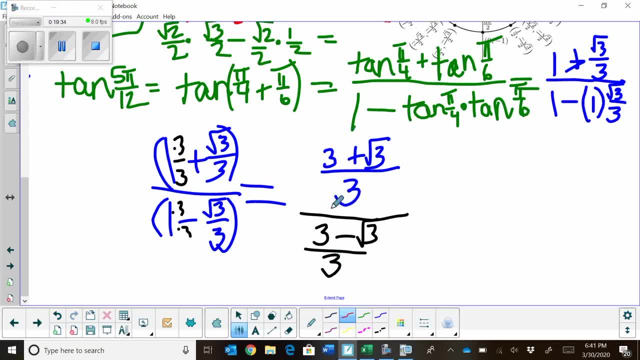 When you have the same denominator in the denominator in this complex fraction, these are the same. You can just cancel them out, right? So you end up with 3 plus root 3, all over 3 minus root 3.. And often you can stop right here. 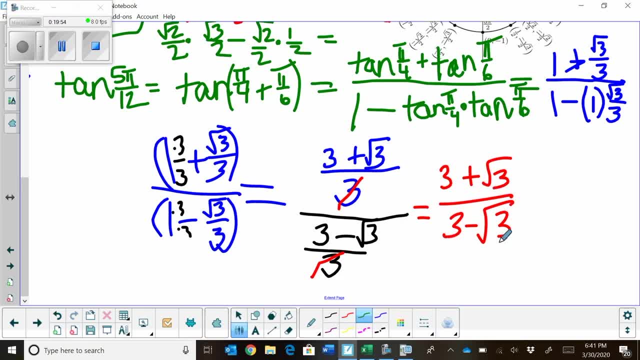 But I beg to differ and I like to clean this up. So I do not have a radical Okay, I have a radical in the denominator Okay. If you remember from Algebra 2 how we handled these, we multiplied these by their conjugates. 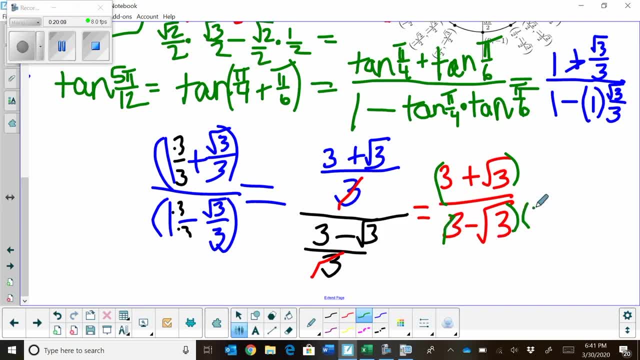 So I'm now going to take this 3 minus root 3 and multiply it by 3 plus root 3.. So I can clean that denominator up to a whole number. Okay, I like to do this for many reasons. One: you just need to know how to do that. 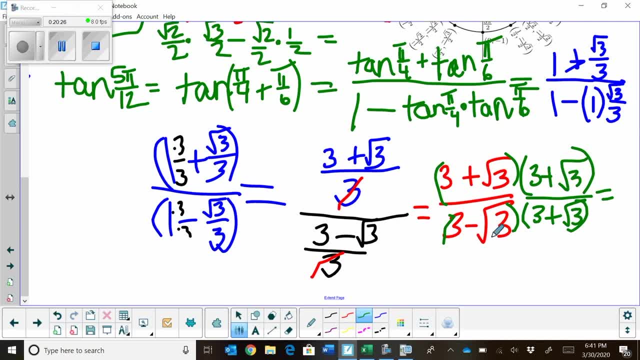 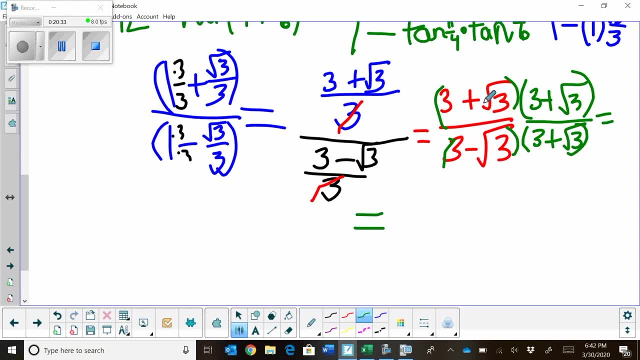 So it just reviews it. You don't ever want to have an irrational number in your denominator, at least at this point in mathematics. Okay, Now let's FOIL this all together. So, first outer, inner, last, do all the multiplying. 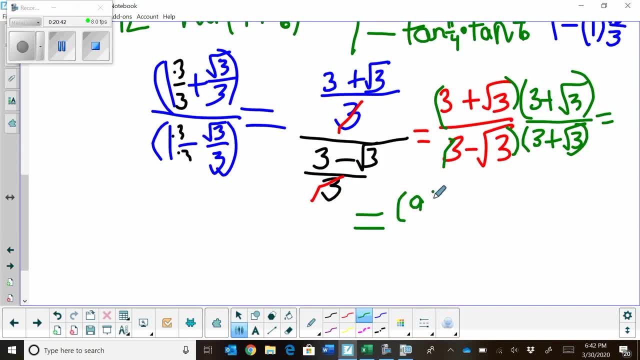 We end up with in the numerator 9 plus 2, square root 3 plus 3, which ends up being 12 plus 2 root 3.. Okay, And then on the bottom we end up multiplying together. First is 9.. 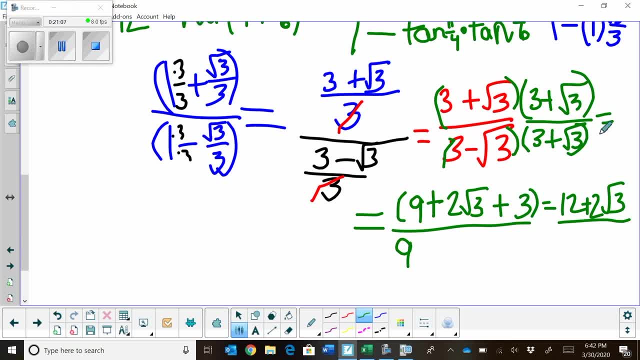 Outer is positive- root 3, or positive 3- root 3.. Inner is negative 3- root 3.. So they cancel. That's what a conjugate does Minus the quantity 3. So I get a 6.. 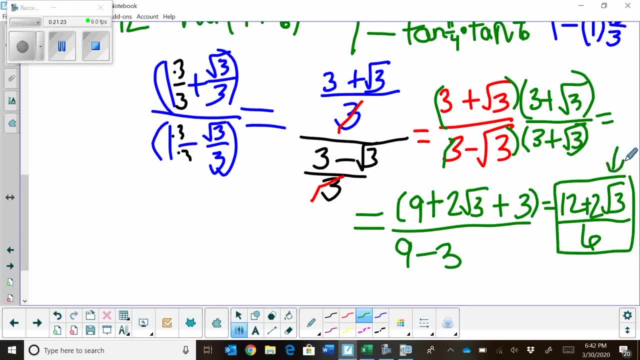 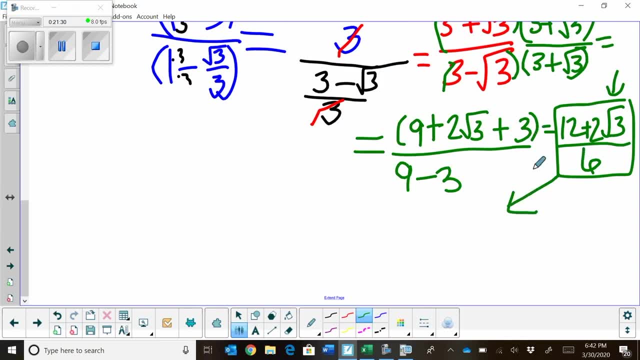 Now this looks like we're almost done, but what are we missing? We can simplify this answer. Okay, So let's go one more step and just divide everything by 2.. So I'm going to get a 6 plus root 3, all over 3.. 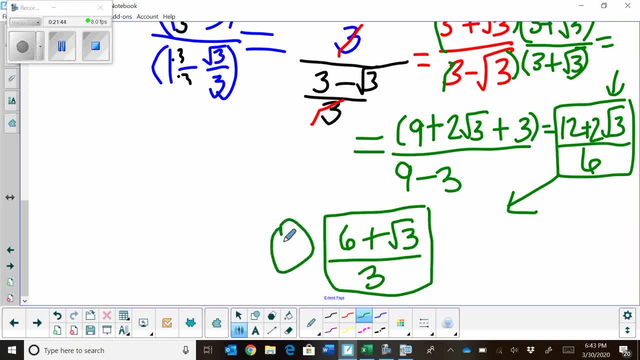 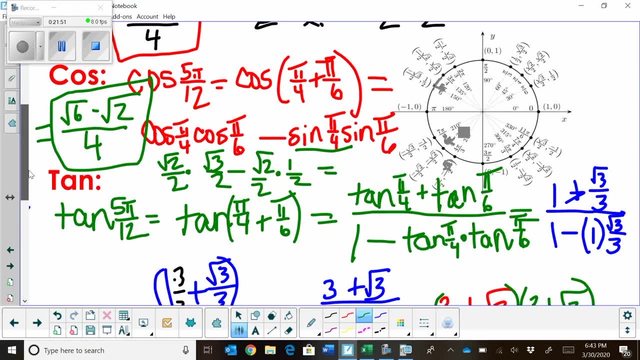 And that, my folks, is our final answer And we finally got there. Okay, So let's look at tangent one more time, because tangent is by far the trickiest. You start with your angle, You rewrite it as the sum of two angles. 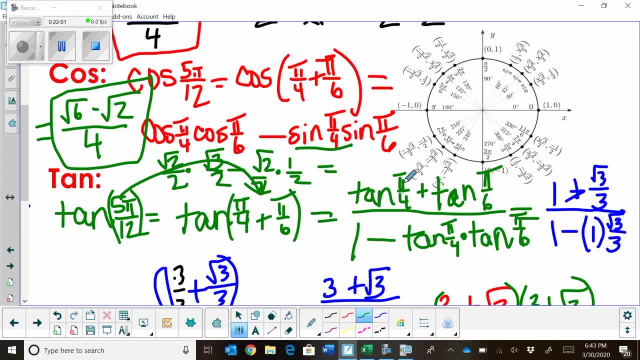 Then you plug it into your tangent formula. Tangent is the sum on top And since this is the sum, the sum is on top of the tangent of the first angle plus the tangent of the second angle over 1 minus their product. Then we plug in: 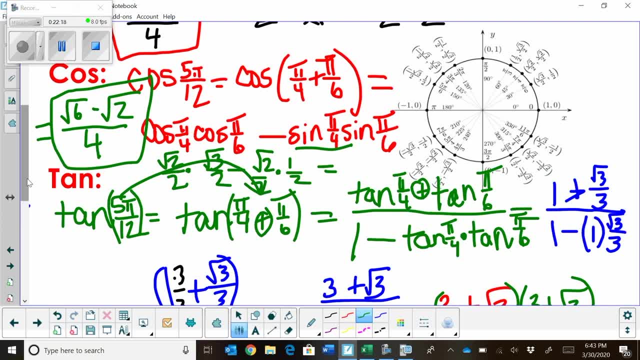 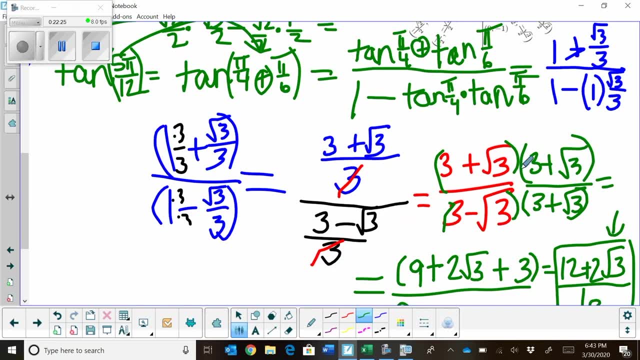 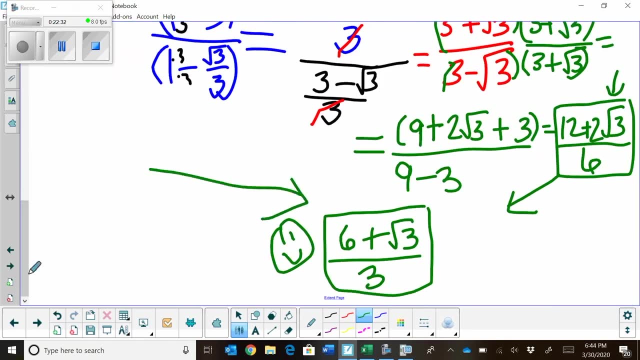 Once we get to here, we just make a complex fraction, So add the numerators together, Add the denominators together, And then we just clean it up. So there you go. That's how we work all the way to this final answer. 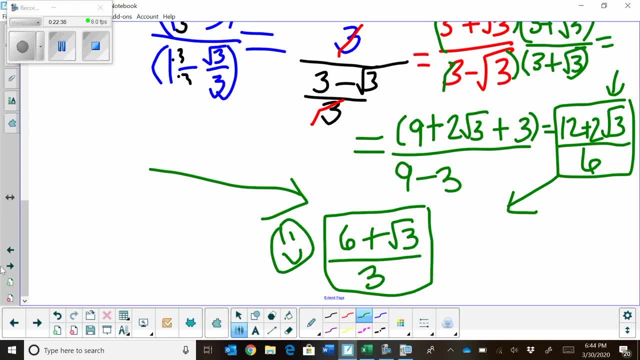 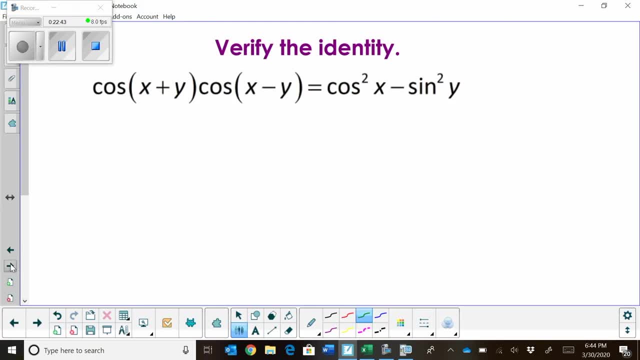 And then, of course, we had to multiply by the conjugate to make it look pretty. So that's just plugging into the values. But there's far more to this concept. We can do identities with these sum and differences. So let's try an identity. 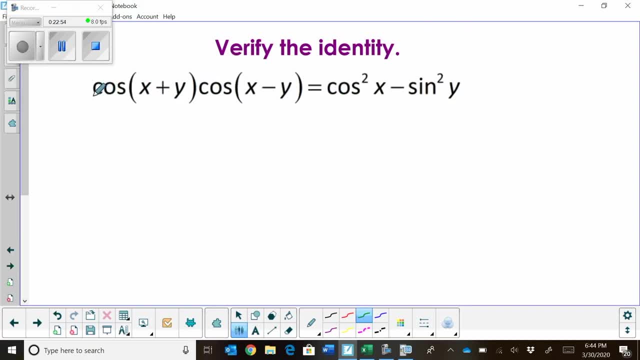 Okay, So we're going to verify this identity, And it's cosine of x plus y times cosine of x minus y. Well, what we have to do is we have to apply the sum and difference of cosine into these angles. So I'm going to expand these out. 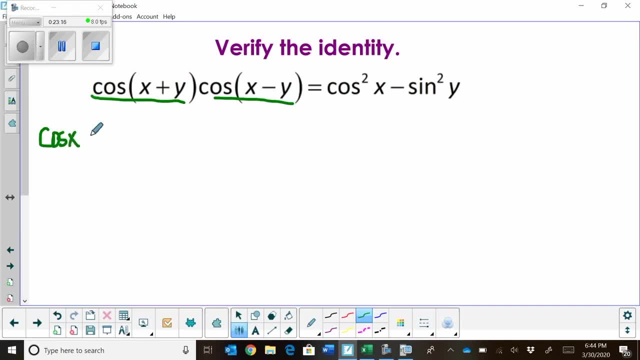 So cosine of x plus y is going to be cosine x times cosine y. Okay, So it's always the opposite sign of sine x and sine y. Okay, So there's my first one. That's the first one expanded. 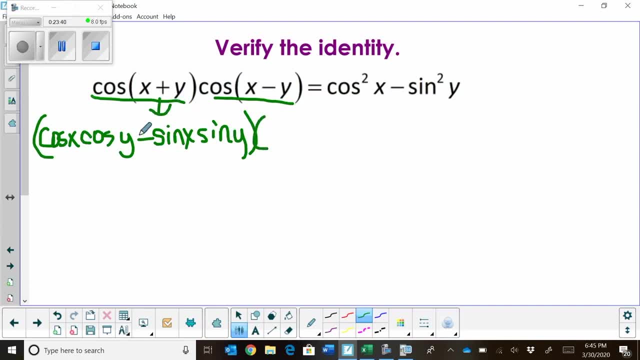 Now let's expand the second one. This is going to look the same, only the sine in the center is going to be opposite right. So I've got cosine x, cosine y, Plus sine x and sine y. Now, once I get to here, what do we do? 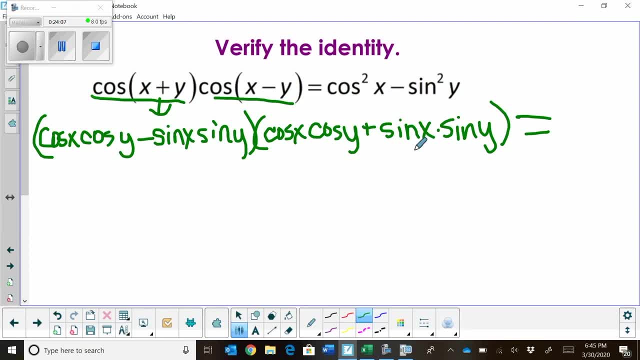 Well, we've got two binomials. So what becomes natural here? Well, what becomes natural is multiplying these together, foiling it. Well, these are conjugates. So you're going to end up first times first And second times second. 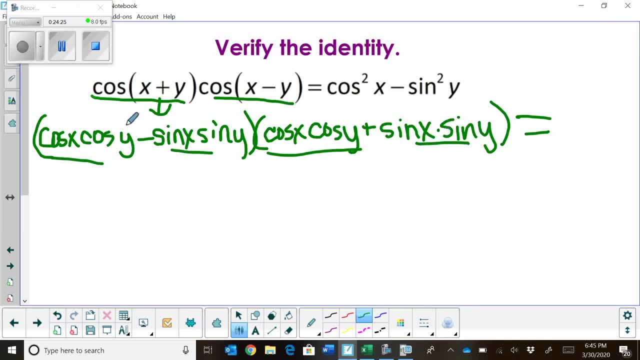 And then the outer and the inner are going to cancel. So let's just multiply first together. So we're going to get cosine squared x, cosine squared y, Minus sine squared x, times sine, Minus sine squared y. There we go. 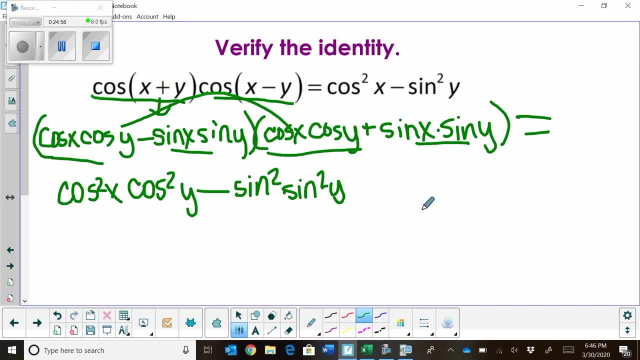 We just foiled that together And this is where we ended up. Hmm, Well, that's not the identity. But is there anything else? Whoops, I forgot my x in here. Is there anything else? we know Well, sine x minus sine y. 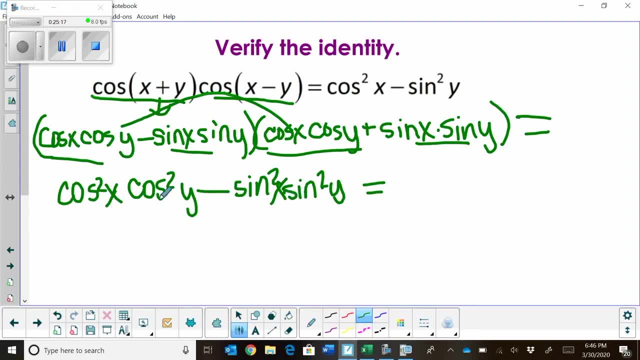 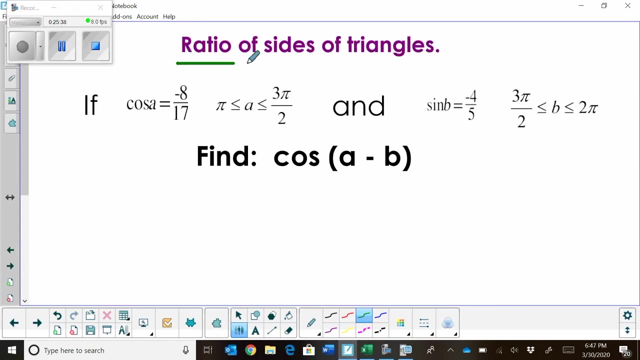 Is there anything we could do here? Hmm, Hmm, I'm not seeing it. I really am not seeing. So we're going to come back and visit this in a minute, Okay, So what's the ratio of two sides of triangles? 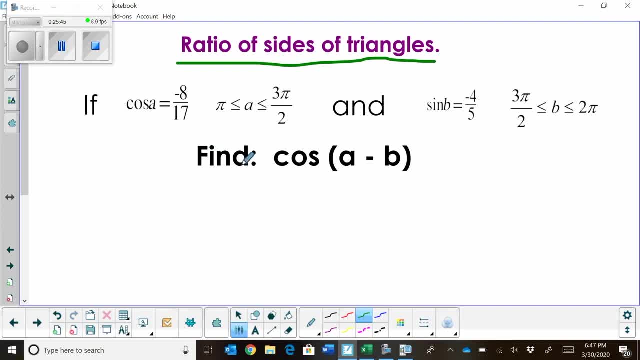 What we're going to do here is we're going to find the cosine of the difference of two angles. When we find the cosine of the difference of two angles, we have to have these angles represented somehow. So what we're going to do is: we've got an angle A. 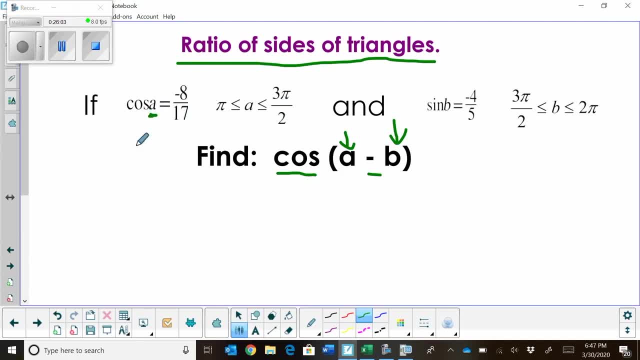 We have a ratio provided And we also have a quadrant provided. So what we're going to do is we're going to draw this triangle in this quadrant. So if cosine of A is equal to negative 8 17ths, we are in quadrant. what? 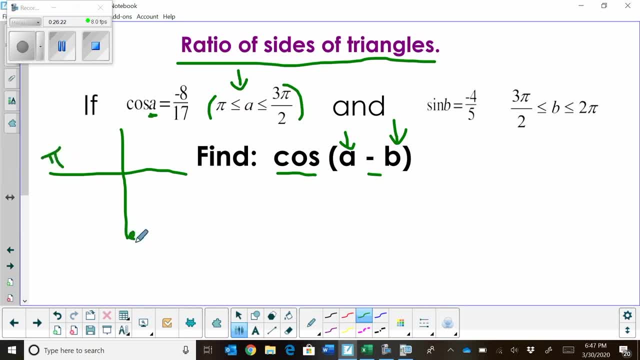 Well, what's pi to 3, pi halves, That's going to be quadrant 3.. I'm then going to draw my reference angle. We know reference angles come out of the origin and go back and touch which axis? The x axis. 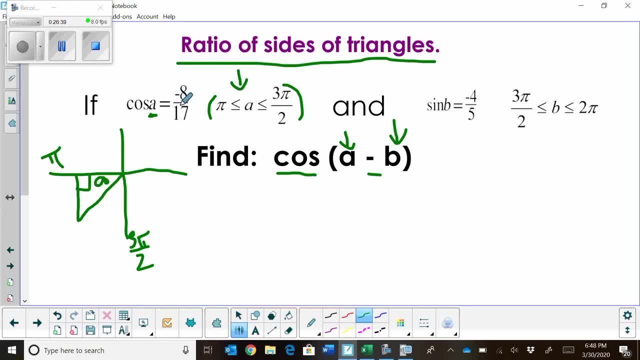 So there's angle A. Now, if cosine is negative 8, 17ths, I'm going to label my triangle with a negative 8 on the x axis, 17 has a hypotenuse And I hope you know your triple. 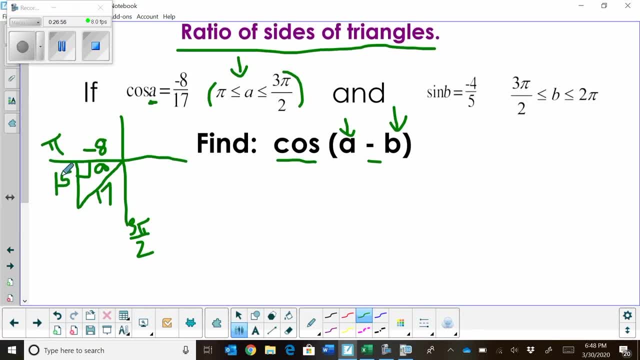 This side will be 15.. Okay, So there's the triangle we're working with, based on this angle A in quadrant 3.. Now, since this is quadrant 3, I know the 15 is also going to be negative, because the coordinates here are negative, negative. 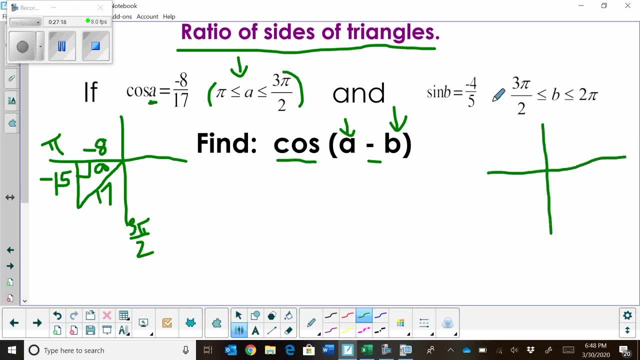 Okay, Now let's look at the second one. Okay, We're looking at the sine of B, So we have a second angle, B And B. we have to draw it. Okay, Which quadrant are we in? We're at 3 pi halves to 2 pi. 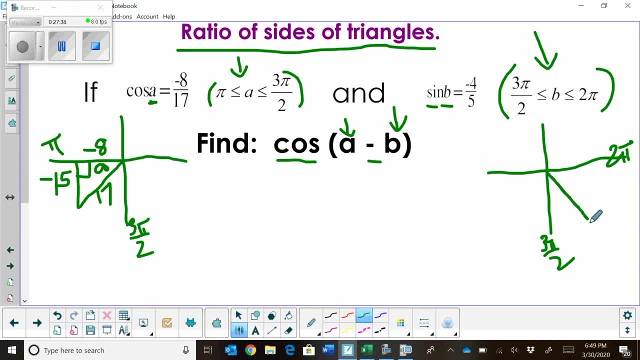 That means we're in quadrant 4.. We're going to draw our reference angle. And what do we know about the reference angle? It comes out of the origin And it touches the x axis, So there's angle B. Now the sine is opposite, negative, 4, hypotenuse 5.. 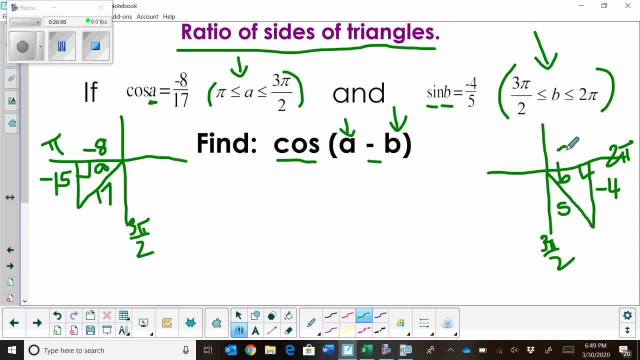 Now, hopefully, you recognize this triple And we know that this direction is 3.. Is that a positive 3 or a negative 3? In quadrant 4.. Well, we know that's a positive 3 because it's the positive direction. positive x direction. 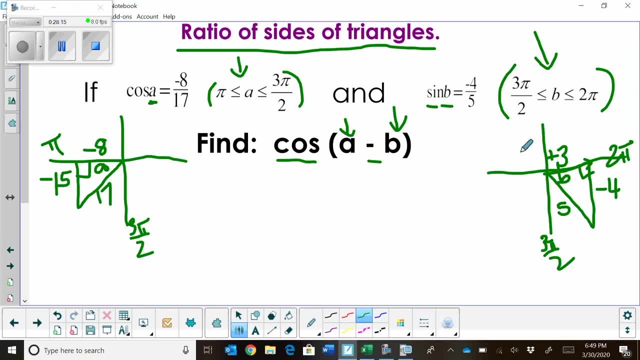 So now that we've got the triangles drawn, the next thing we're going to do is expand this out. So for cosine, we need to know that it's cosine A, cosine B, opposite sine. So plus sine A, times sine B. 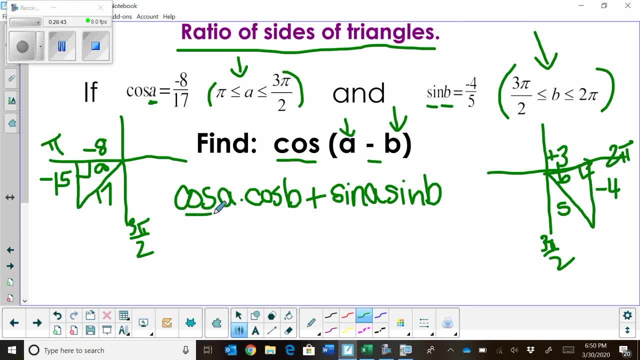 Now we're going to use our triangles to evaluate all of these. Okay, So let's start with the cosine, Cosine of A. Well, cosine of A was actually given to us. It is negative 8 17ths. 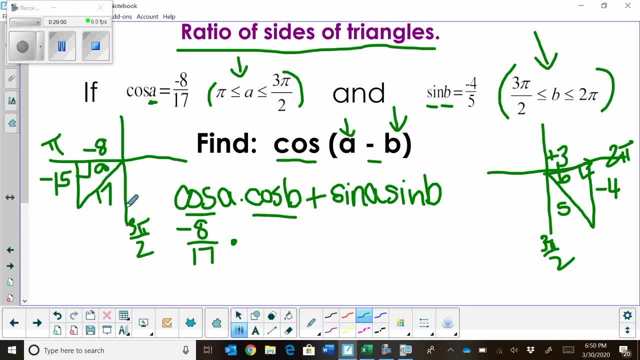 And that makes sense because it's adjacent over hypotenuse. We're going to take that and multiply it by the cosine of B. Well, this is B, And what do we know? cosine is here Adjacent over hypotenuse, So 3 fifths plus sine of A. 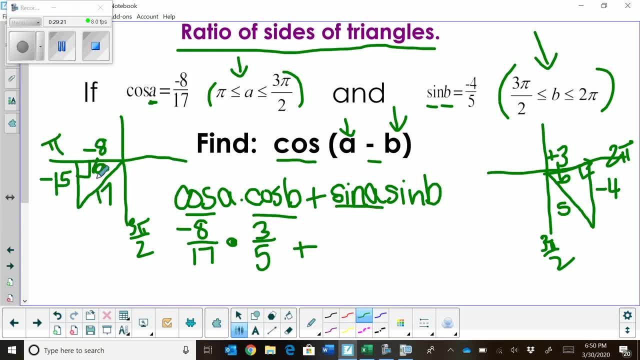 So we're going to go back to the first triangle because that's angle A, The sine is negative 15, 17ths And we're going to multiply that by the sine of B, So go back to the B triangle And sine of B was given to us. 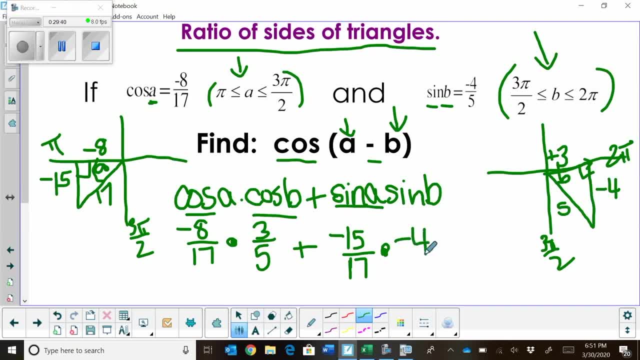 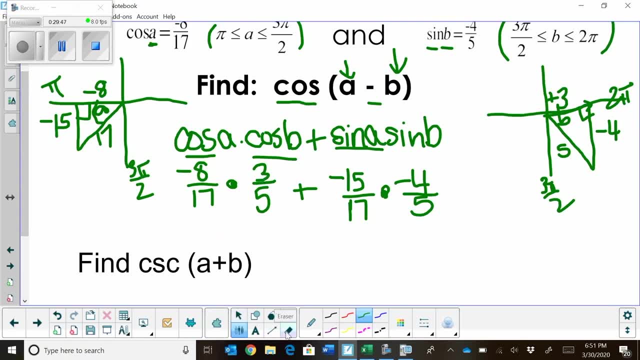 It was negative 4 fifths. And there we go Now. we just need to clean this up. So whoops, I'm not quite ready for cosecant yet. I'm going to multiply this together and I get negative 24 on top in the numerator. 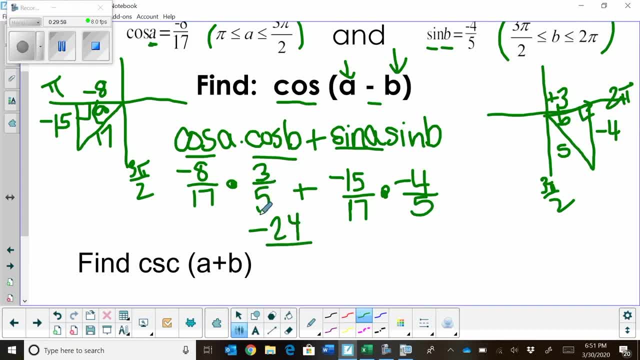 And 5 times 17.. 5 times 17 is 35.. Carry the 3.. So what's that? 85. Okay, 85 plus, And then a negative. times a negative is a positive And 4 times 15 is 60 over. 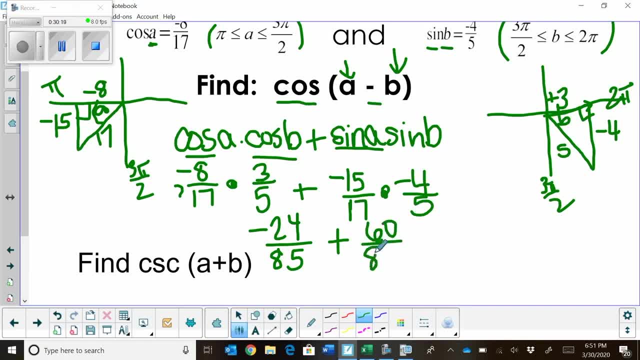 And then again, 17 times 5 is 85. And now they have a common denominator. So all I have to do is subtract And 60 minus 2. 24. That's going to give me 36 85ths. 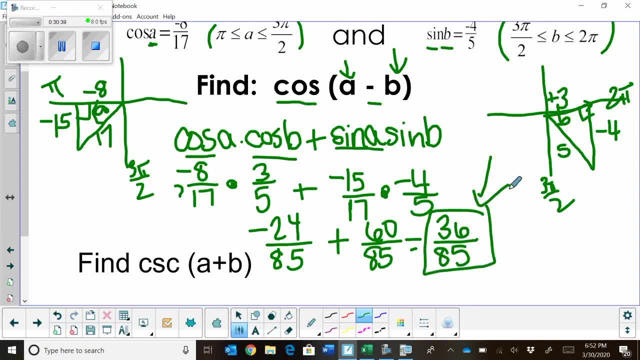 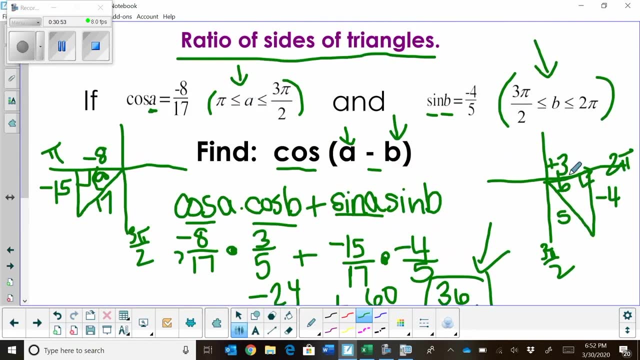 And that is my final answer, That's the cosine of A minus B. Wow, That's a lot Okay. So what did we do? We wrote out the first. We drew the triangles right In the correct quadrants. 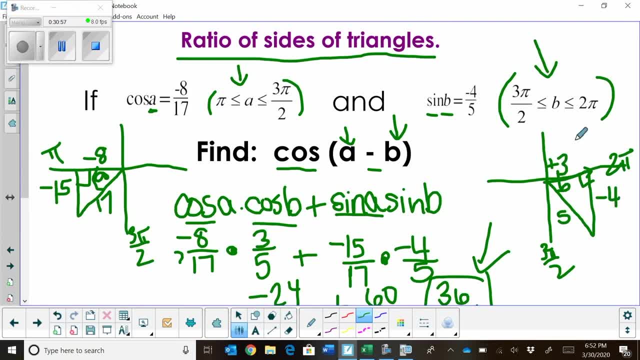 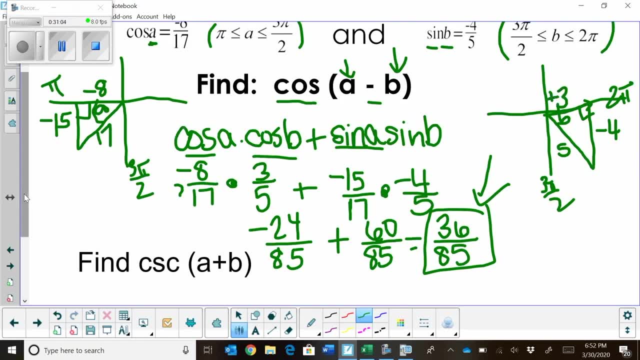 Making sure our signs S-I-G-N are the right quadrants. Then we wrote out the cosine formula and plugged it in, based on which triangle we were using. Now what would we do if we're finding the cosecant of the sum of two angles? 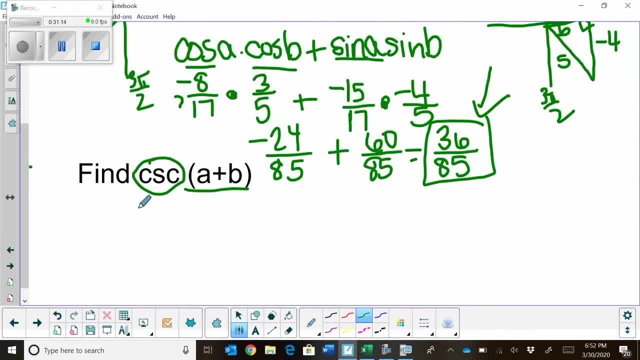 Well, I hope you're thinking. well, there isn't cosecant formula, But we do know a sine formula And we know the sine and cosecant are reciprocals. So what we're going to do is we're going to evaluate this as a sum. 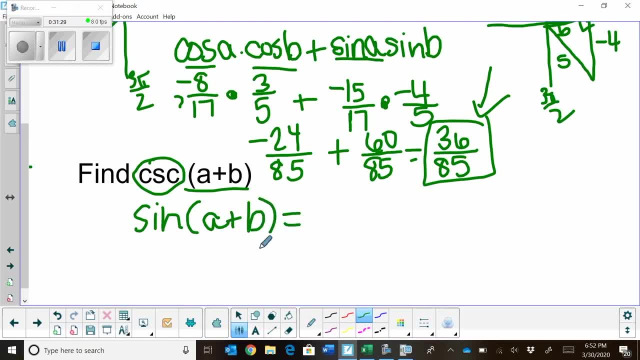 As a sine, As a sum of two angles of sine. Then we're going to take the final answer and we're going to find the reciprocal. So let's write out the formula for sine. It's sine A times cosine B, Same sine. 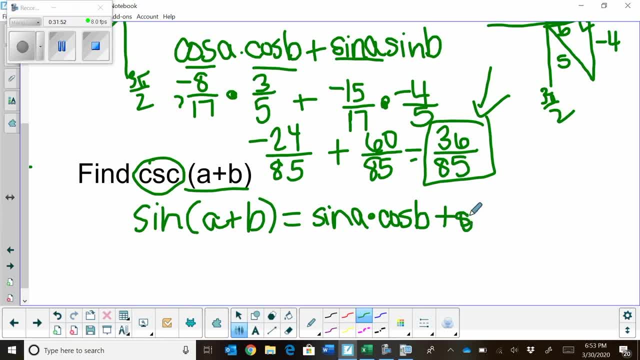 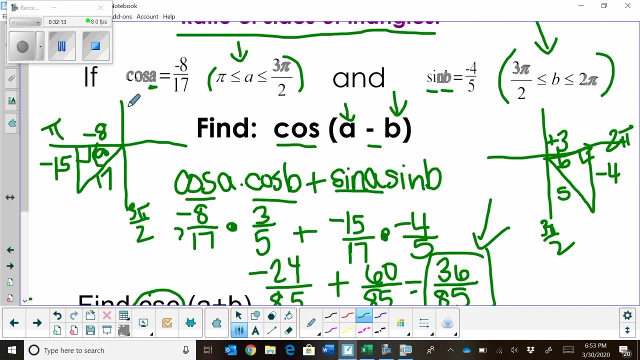 So adding sine- I'm sorry- Cosine A Times sine B. So it's sine cosine, cosine sine, Same sine. Now let's go back up and evaluate. So the sine of A, Here's the A triangle. 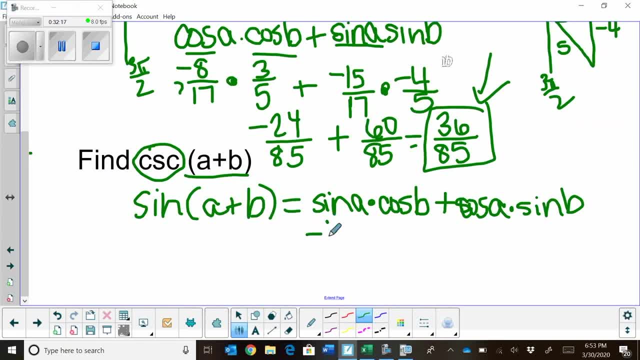 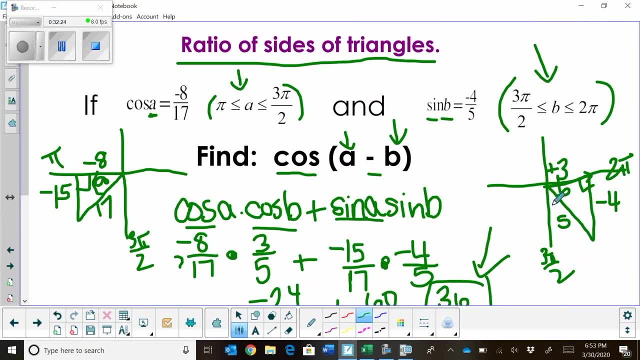 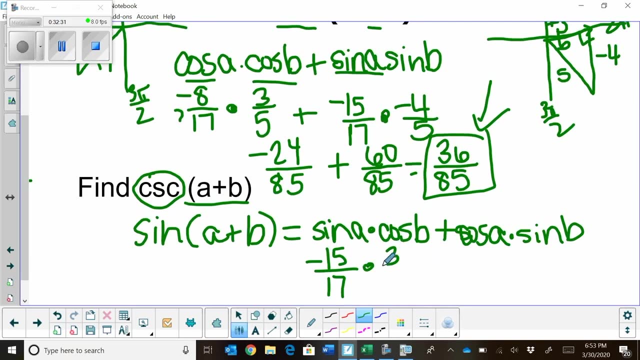 And the sine is negative: fifteen-seventeenths Times the cosine of B. Well, let's go to the B triangle. Mind the cosine. The cosine is three-fifths, So times three-fifths, Plus the cosine of A. 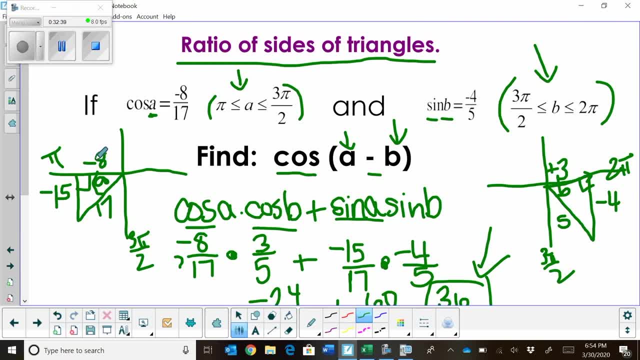 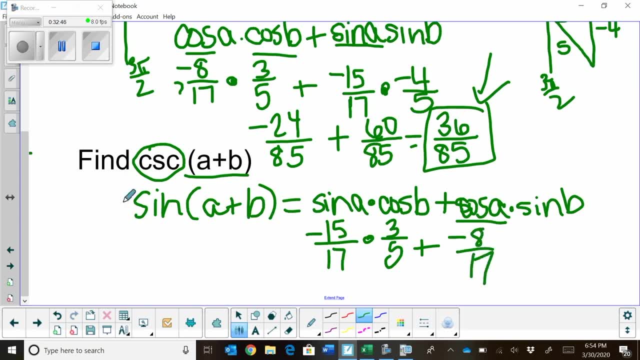 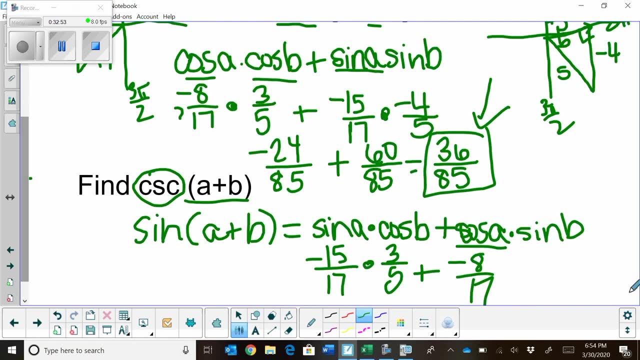 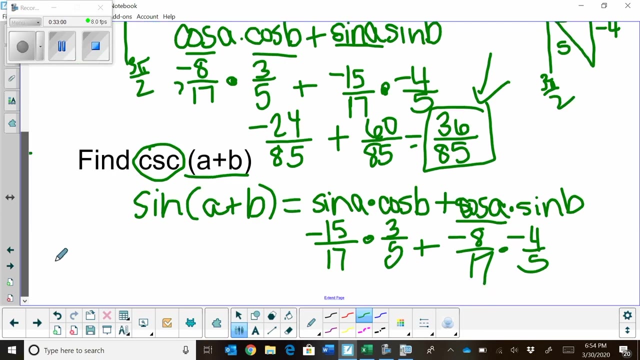 Let's go back to the A triangle Cosine is negative eight-seventeenths. That was given Times. the sine of B, Sine of B is negative four-fifths. That too was also given. Now let's just evaluate or simplify those. 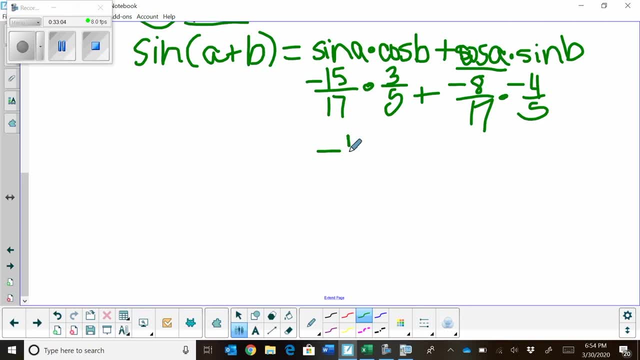 And that's going to give me negative. forty-five over eighty-five, Plus two negatives make a positive, So thirty-two over eighty-five, Same denominator. So that makes it nice. What's our difference? It's thirteen, So negative. thirteen over eighty-five. 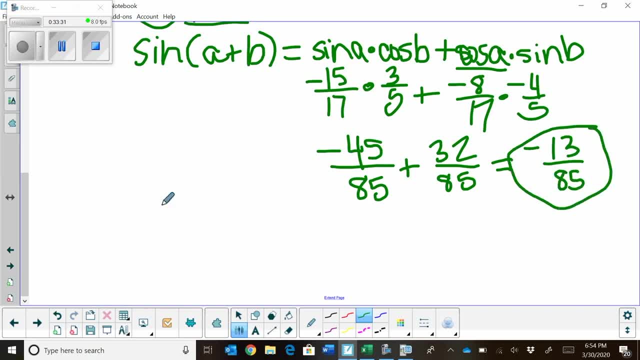 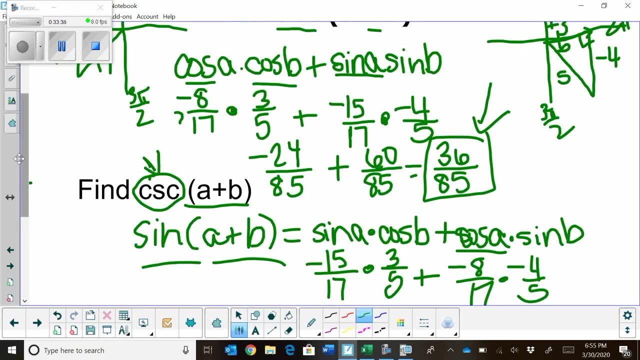 And that, right here, is my sine of A plus B. Now, we didn't want the sine. What did we want? We wanted the cosecant. So what are we going to do? We're going to take its reciprocal. 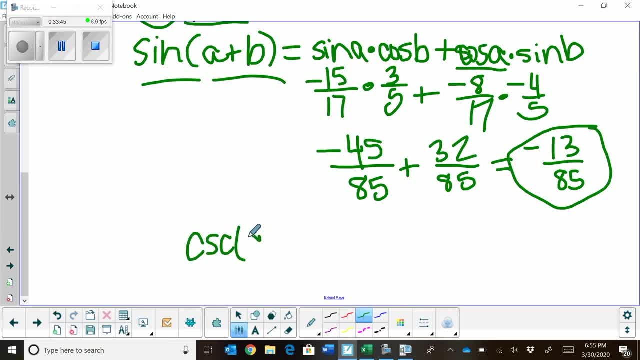 So the cosecant of A plus B would then be negative. eighty-five, thirteenths, And there's our answer. So yes, I have the negative with the thirteen And you can write it as eighty-five over negative thirteen. 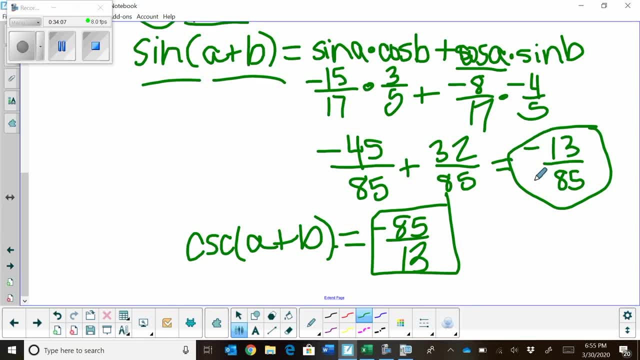 But typically we just keep the negative with the numerator up top, Because the term is negative, That's just a term. So there we go, And that's how you'd evaluate those sums. Okay, So this is actually a step back. 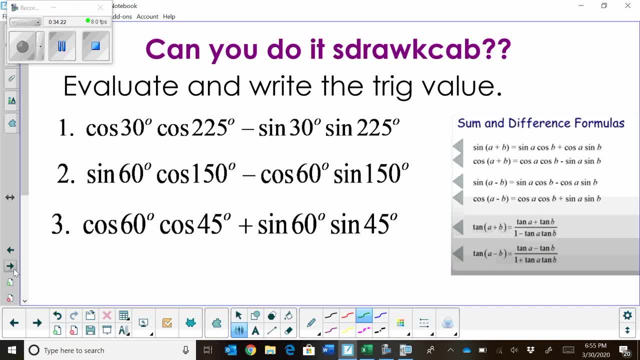 Makes it a little easier. Can you do this? Do you recognize that word? Can you do it backwards? Yes, Can you do it backwards. This is the word backwards that's written backwards. Can you do this backwards? In other words, can you look at an expansion, decide which equation it is? 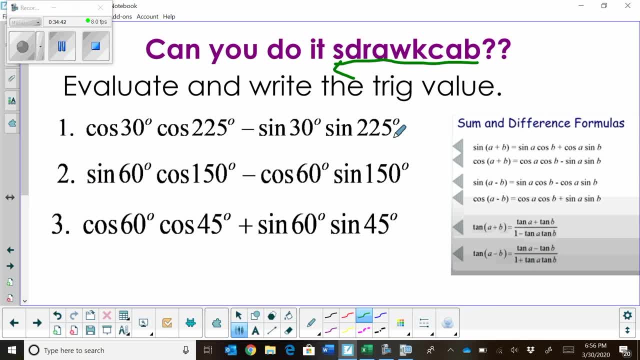 Is it the cosine, Is it the sine, Or is it the tangent? Do I add, Do I subtract? What would it look like? Okay, So let's look at the first one. We have cosine thirty, Cosine two twenty-five, minus sine thirty, sine two twenty-five. 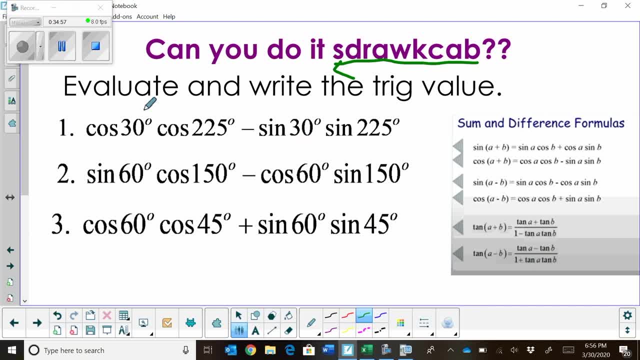 Well, is this the cosine or the sine formula? And I hope you're going: oh, cosine, cosine, sine, sine. That's the cosine. Yes, indeed, that is cosine, But when you expand it, it's always the opposite: sine. 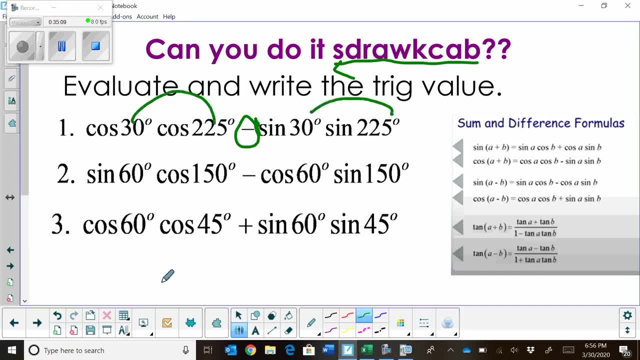 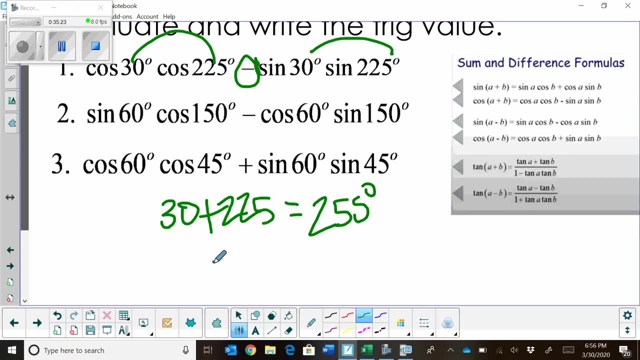 So we're going to end up adding these two angles together. So thirty plus two twenty-five. That just adds to what's that? two fifty-five, Two fifty-five. So really, what are we evaluating? We're evaluating the cosine of two fifty-five. 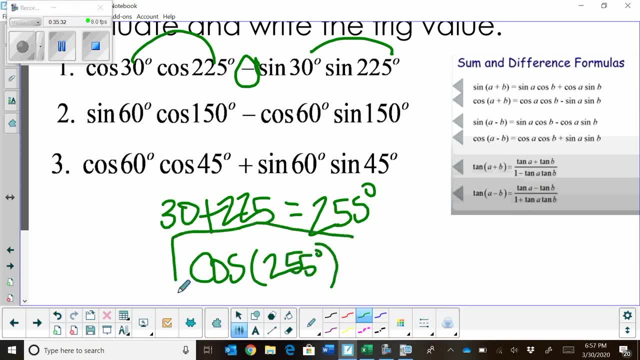 That's all we're doing. We're looking at the formula, seeing if it's the sum or the difference, and then like squeezing it back together and deciding what it is. So let's look at the second one. The second one is: sine sixty, cosine one fifty, minus cosine sixty sine one fifty. 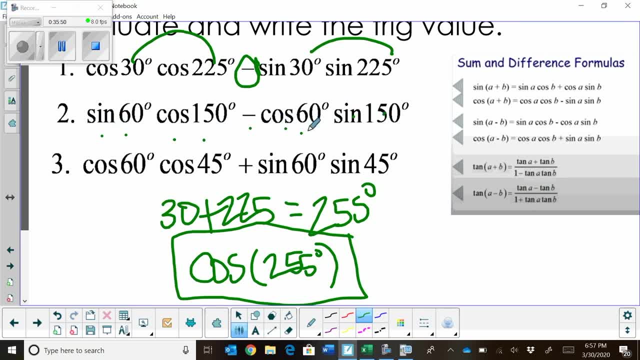 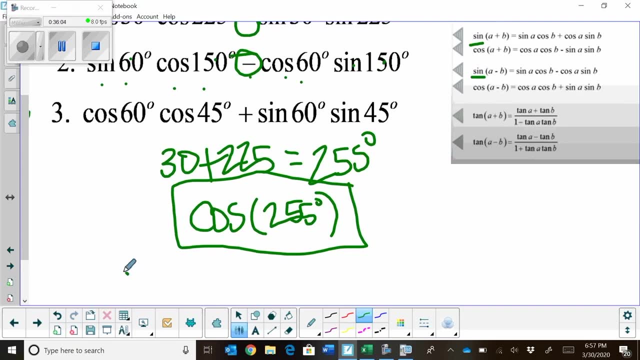 Okay. Well, looking at this, we know it's the sine formula. So sine keeps the sine. So it's going to be A minus B. Don't be tricked, Be very careful. This is the sine of the A angle. 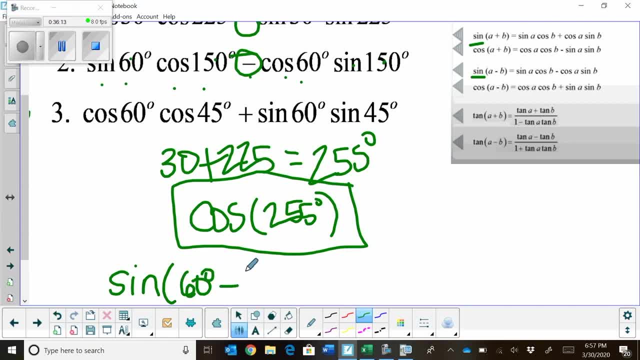 Angle A is sixty minus one fifty, And sine keeps the sine. So we are indeed going to subtract. We're going to subtract those two, So it's going to be the sine of sixty minus one fifty. That's negative ninety. 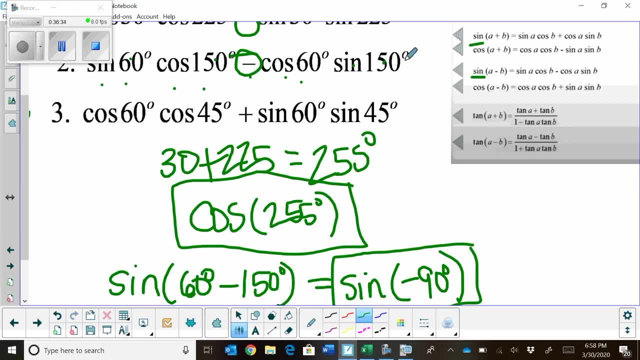 So, yeah, it's okay that it's negative, That's okay. Okay, So that's where this one comes from. Okay, Now let's go back, do a little racing so we can look at this last one and have our. 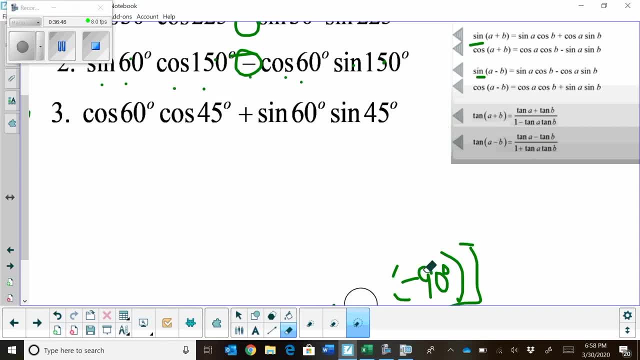 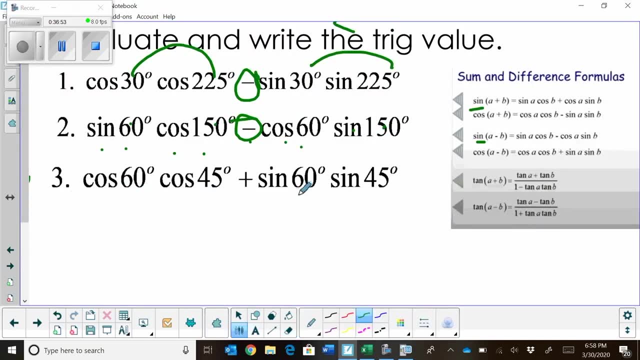 formulas right here on the same page. Now we need to look at this last one First. is it a sine or a cosine formula? Cosine, cosine, sine sine. I hope you're going. oh yeah, that's cosine. 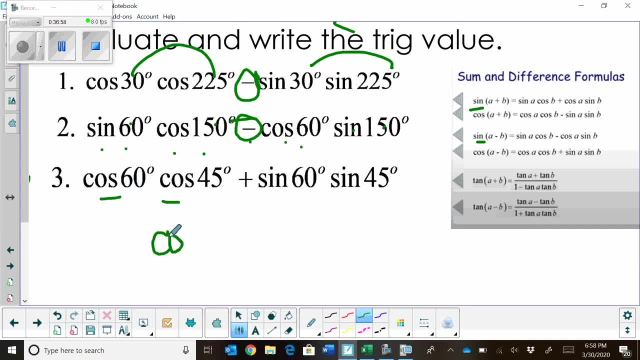 Okay, cosine, And that's going to be. the two angles are sixty and forty-five. Now I want you to think: Okay, cosine, it's addition here. but what do we know about cosine? It's always the opposite sign. 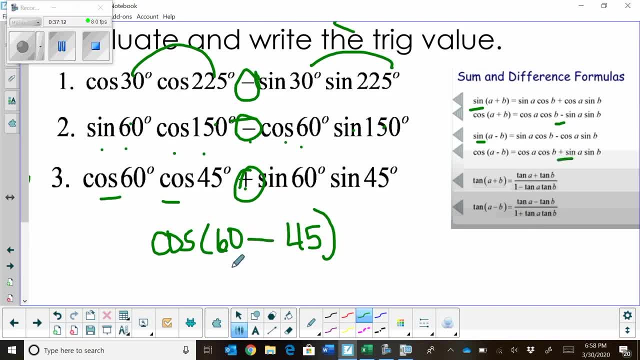 So we're going to subtract: So sixty minus one fifty. So sixty minus forty-five is cosine of twenty-five degrees. Bingo, Right? No, no, no, no. Fifteen degrees, Yeah, it's just fifteen degrees. 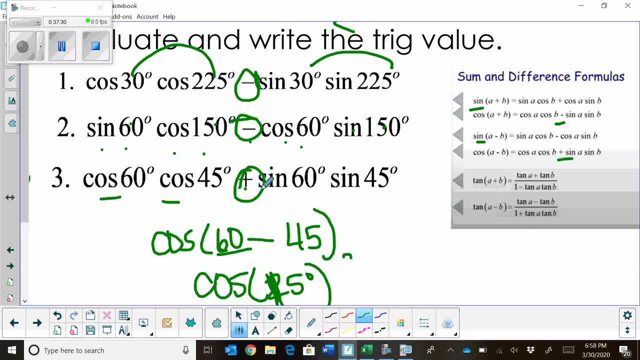 Sixty minus forty-five is fifteen, So it's a cosine of fifteen. So you could evaluate the cosine of fifteen with this expansion. And there is our answer. And that's all we're looking for is to condense it back together. 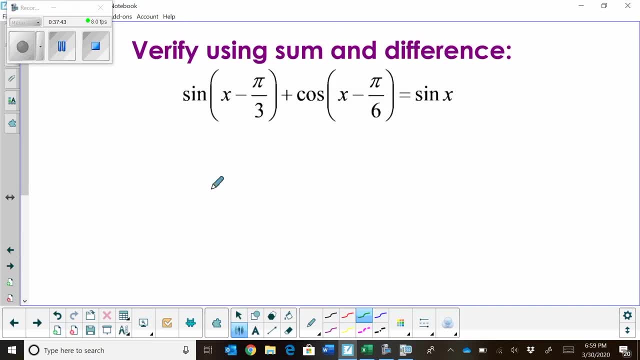 Now verifying- Okay, Verifying- a second identity. Let's go ahead and try this one. I really like these. These expansions make a little more sense. Okay, we're going to verify this identity by expanding a sign and by expanding a cosine. 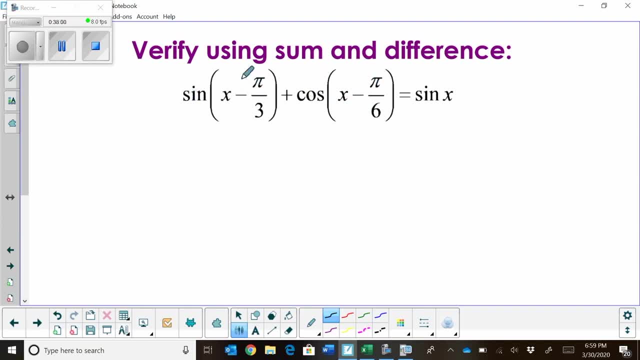 Okay, they're both a difference. but we know that sign will keep the negative and cosine is going to change that to a positive. So let's expand these, Okay. Cosine of x times cosine of pi-thirds: Same sign, so minus cosine pi-thirds times, I'm sorry. cosine of x times sine of pi-thirds. 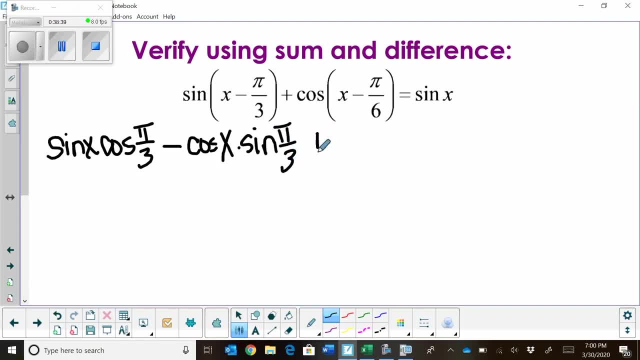 Okay, we're going to take that. We're going to add to it this expansion. This expansion is cosine times cosine, So cosine of x times cosine of pi-six. Now we need to change this sign, So it's going to be another addition sign. 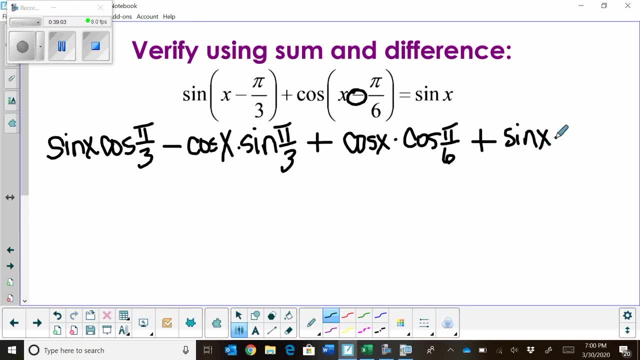 Sine of x times sine Sine of pi-six. Now let's evaluate the ones we can. We know that cosine of pi-thirds we can evaluate Sine of pi-thirds, and then cosine of pi-six and sine of pi-six. 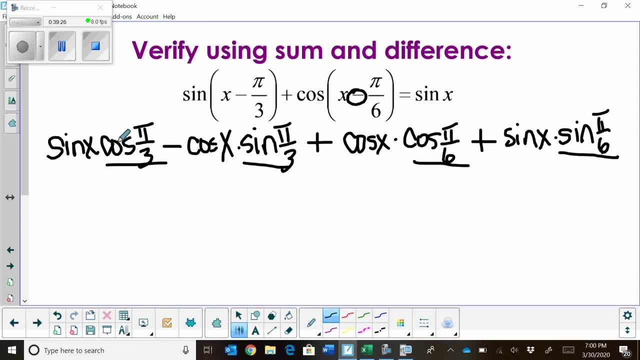 All those can be evaluated. So we're going to have a coefficient that's then going to go in front of this. So what is the cosine of pi-thirds? Well, that is a root. I'm sorry, cosine of pi-thirds is a half. 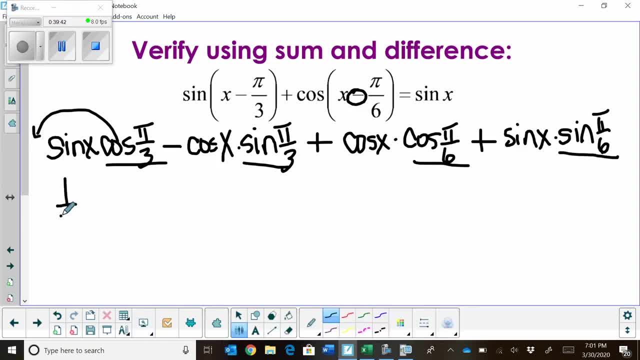 One half of sine x Minus the sine of pi-thirds is a root three over two times cosine of x Plus Cosine at pi-six. That's a half right. No, that's a root three over two. It's late in the day. 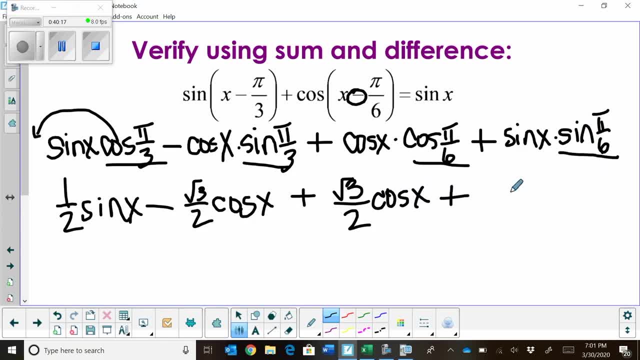 And then plus sine of pi-six, That's just a half Sine x. Okay, so let's look and see what we have. We have a half of sine x. Negative root: three over two. Negative root three over two. Cosine x. 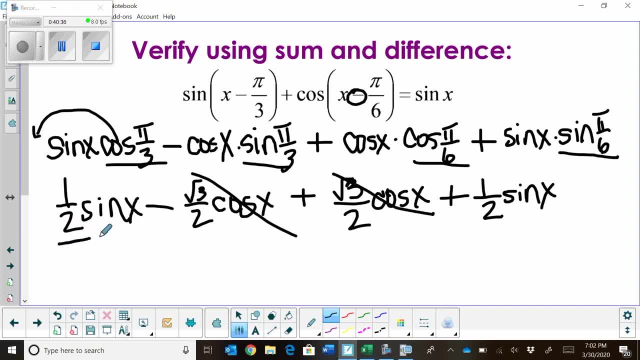 Positive root three. Oh, these cancel. Then I have a half sine x, A half sine x, A half and a half make one whole Sine x. That indeed equals sine of x. So bingo, We did it. And there is verifying that sum and difference. 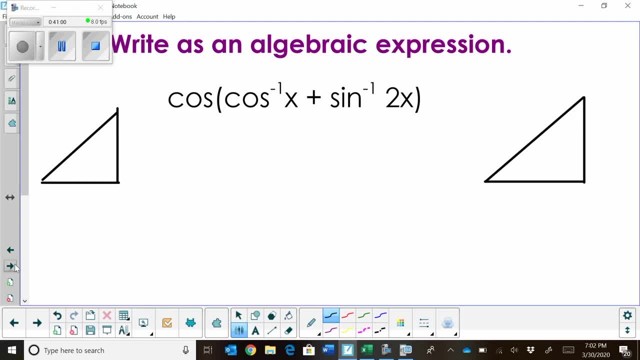 Okay, So Let's take one more little stretch. here We're in the home stretch. Okay, Hang in there with me And you can take a break any time you need to, But we're going to evaluate the cosine of these two angles. 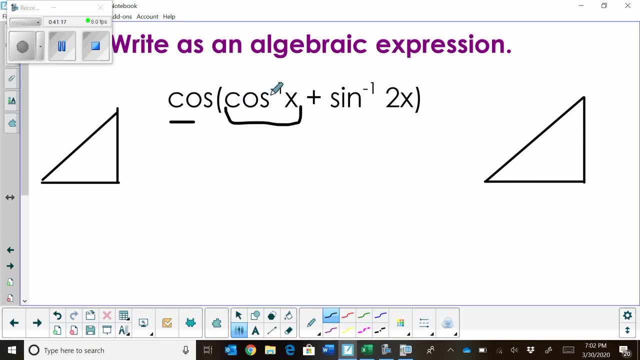 So I want you to think for a second. When you take the inverse of a ratio, doesn't this represent an angle? And the inverse of a sine of two x, that's an angle. So we're taking the cosine of an angle plus an angle. 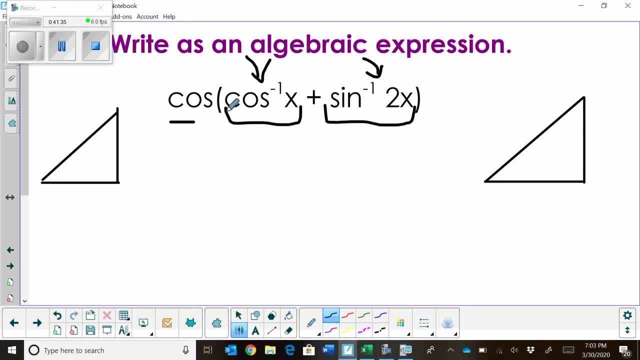 So this is the sum of two angles. Okay, Well, let's write this angle out in the triangle. So I'm going to use this as my angle, My reference angle. We'll call that theta one. Okay, So theta one. 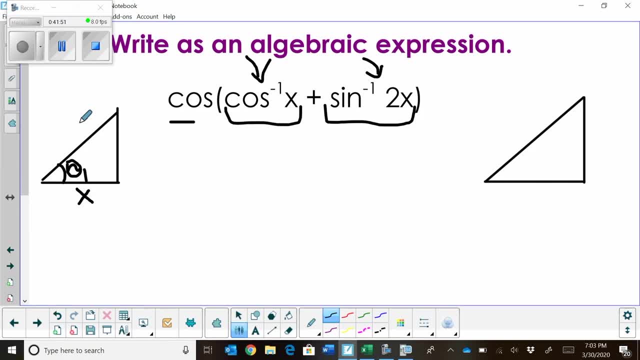 My cosine is x. That means this is x. My hypotenuse must be one. And what did we learn? We learned in one of the other units that the opposite side- we're going to use the Pythagorean theorem- I'll call this side- that we're looking for b for a second. 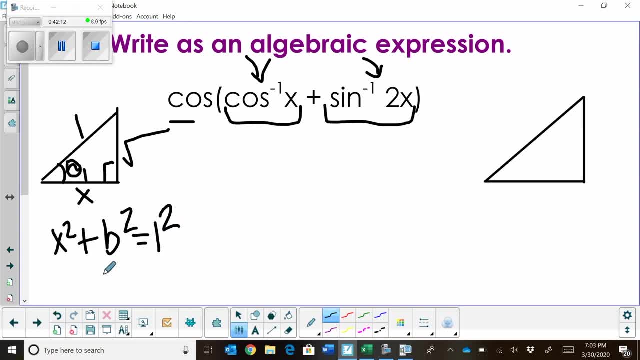 Okay, It's equal to one squared Pythagorean theorem. So b squared is equal to one minus x squared. So this side b is equal to either plus or minus one minus x squared. Now if we're not given a quadrant, we're going to assume we're in quadrant one. 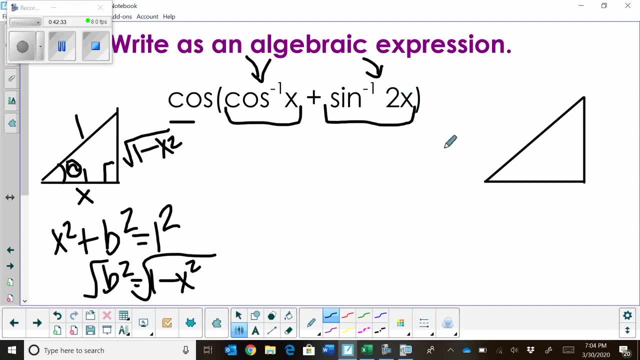 So there's our first triangle. We're going to do the same thing over here, The second angle. So this is like theta two And this is theta one. We don't know the angles, but we know we've got a ratio of those. 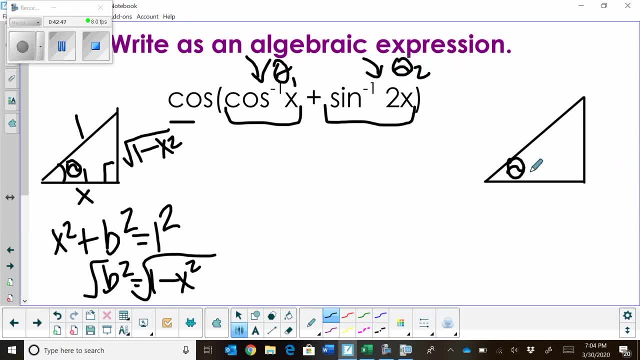 Okay, So theta two, We have a sine, And for sine- that's your opposite- over your hypotenuse. Well, the hypotenuse must be one. So what do we know? this adjacent side is using the Pythagorean theorem. 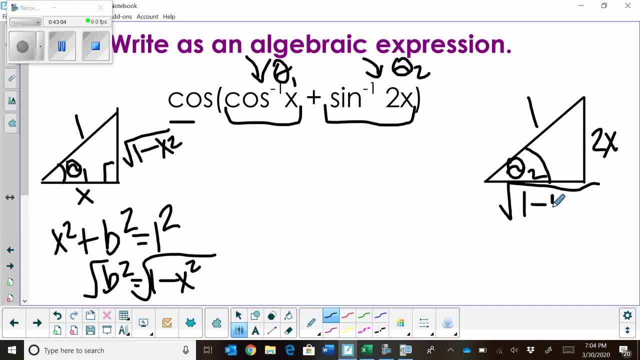 It's one. It's the square root of one minus four. Remember the four? We had to square that x squared. If you couldn't remember that, you can do well. a squared plus two x squared is equal to one squared. 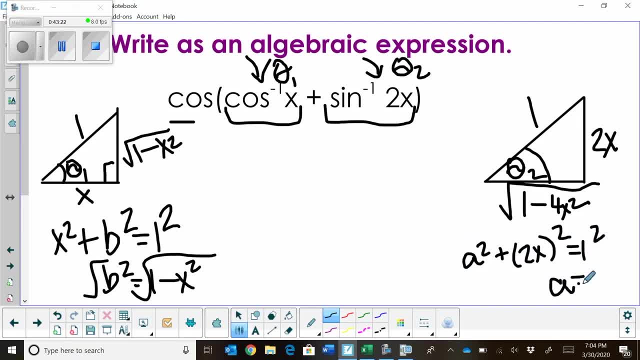 And then work from there to get a, And the a ends up being one minus four x squared, And then you have to take the square root of all that. So that's where it comes from. Okay, So now we have our triangles drawn. 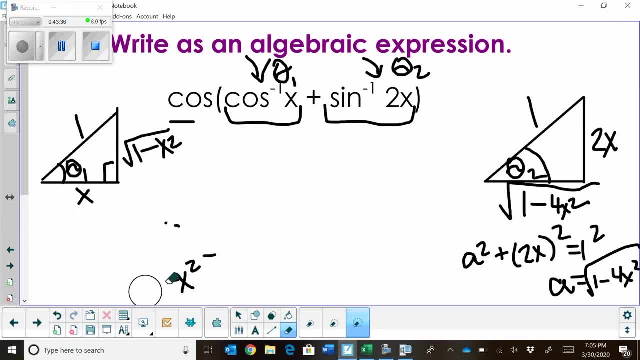 Now we need to expand the cosine formula, So it's going to take a little bit, So we have to take: cosine is cosine of the first angle. I'm going to call this theta one. Oops, Theta one times cosine, theta two. 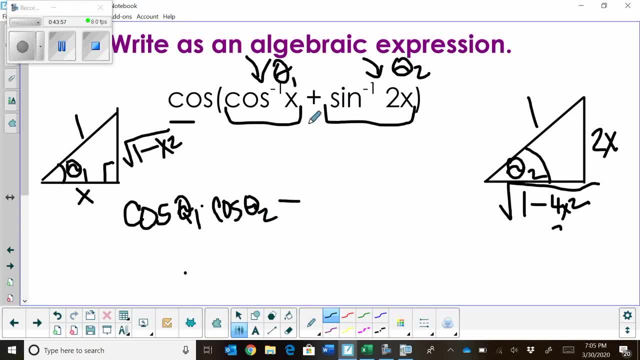 Minus because it's opposite sine Sine theta one and sine theta two. Now let's plug in what we know. Cosine of the first angle is just x times cosine of the second angle is root one minus four, x squared. 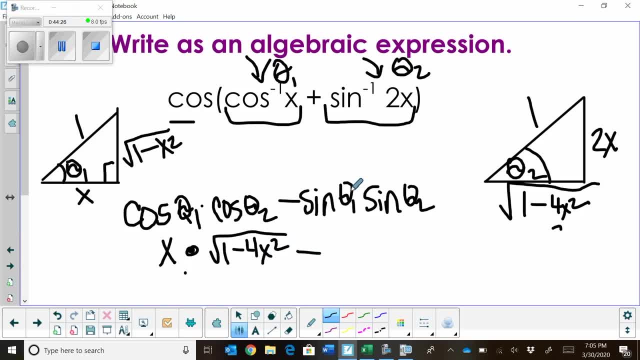 All minus sine of the first angle. Well, that first, the sine is opposite over hypotenuse. So one, the square root of one minus x, squared All times the sine of the second angle, which is two x. So what do we end up with? 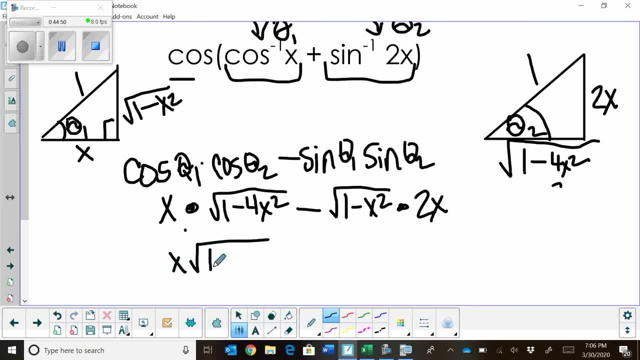 We have x root, one minus four x squared. All minus two x, because I'm going to put my monomial in front of my radical. One minus x, squared. Now, the radicals don't match. So we're done. That's all you can do. 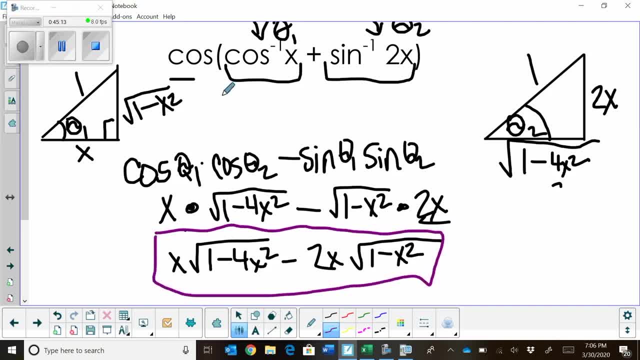 That's as far as it will simplify, And that is the cosine of these two angles, the sum of these two angles. There's our final answer. Easy, isn't it? Okay? So we've done all kinds of stuff. We've done verifying. 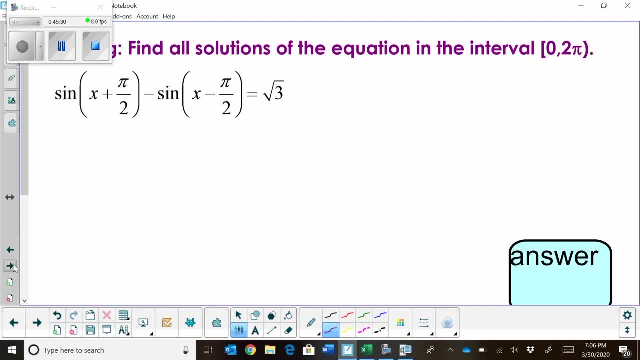 We've expanded those formulas. Now let's use expansion to solve: Whew, We're going to solve it now. So we've got this equation. We're subtracting a sum and a difference to get root three. So guess what we have to do? 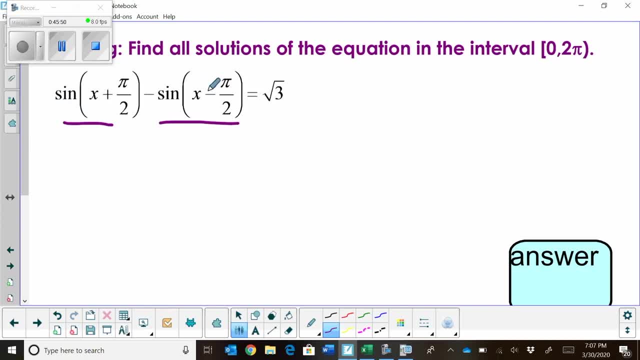 We have to expand both of these out, Collect our like terms and then evaluate. So let's start expanding. Sine, we know, is sine, cosine, same sine. So we're going to add cosine and sine. Okay, So first half we're done. 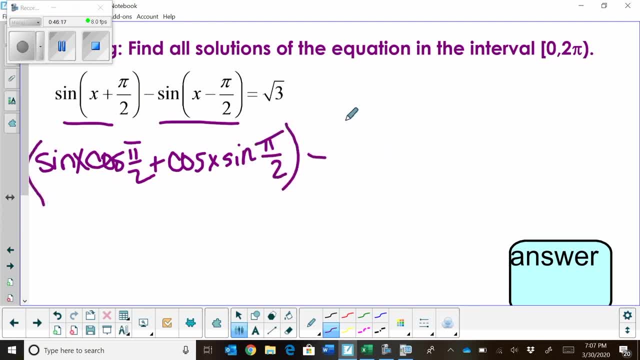 That's the first expansion. Then we're going to subtract the second whole expansion. Well, this one's sine x, cosine pi halves Same sine, So minus cosine pi halves sine x. So that's a lot of stuff, And then that's all equal to the square root of three. 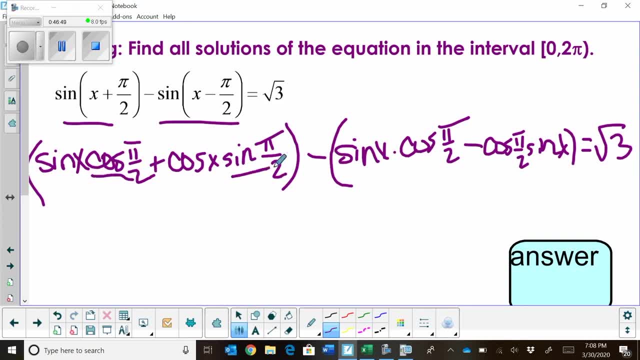 Now let's evaluate what we can. Well, we can evaluate all the ones. We can evaluate all the ones that are sine and cosine of whoops, of whoops. I've got that last one backwards. Y'all didn't catch me. 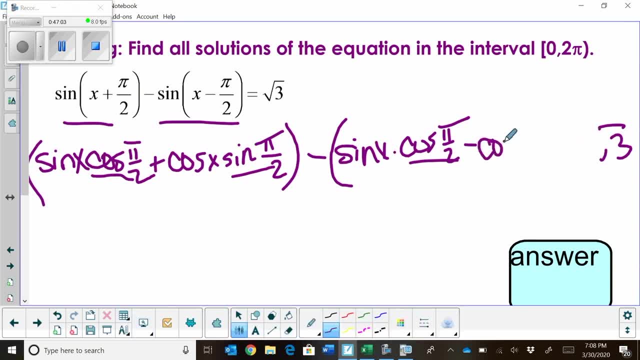 Let's fix that one. So this is going to be cosine x, sine pi halves. See, when I'm not in the classroom, there's no one to catch my mistakes. Okay, So now let's evaluate the four terms we can evaluate. 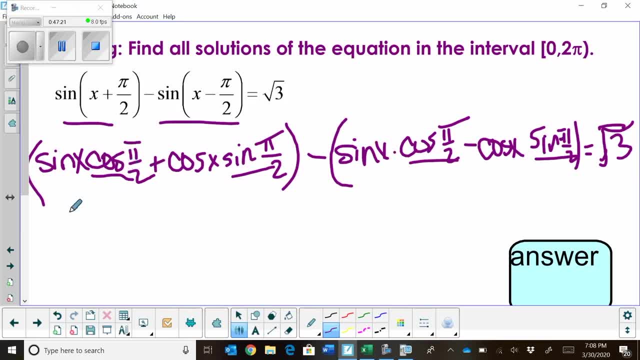 Well, what's cosine of pi halves? Well, that's zero. So we've got sine x times zero. That's just gone because that's zero. And then we have cosine x times sine at pi halves. What do we know? sine at pi halves is: 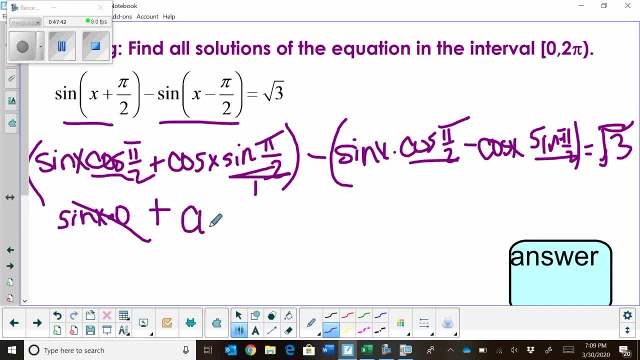 One. So one times cosine x is just cosine x. Well, that turned out nicely. This whole side ends up just being cosine x. Now we're going to subtract this entire quantity, so we have to be careful. Sine x of cosine of pi halves. 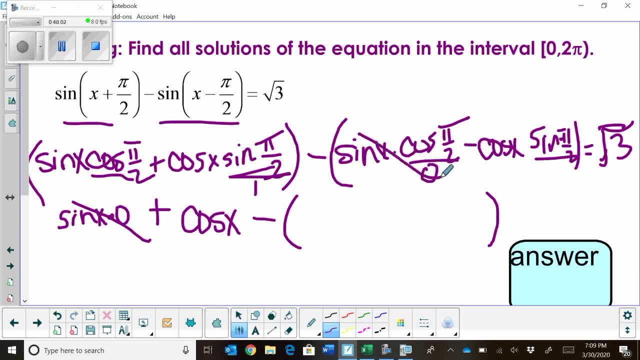 Well, didn't we just say: cosine of pi halves is zero? So this part is gone. And then we have minus cosine x times sine of pi halves, which is one, So we have a negative cosine x inside here. Okay, 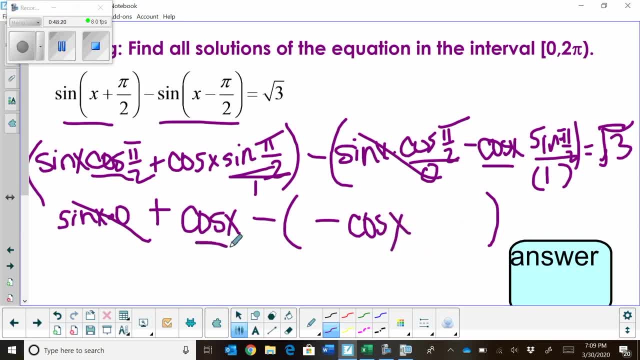 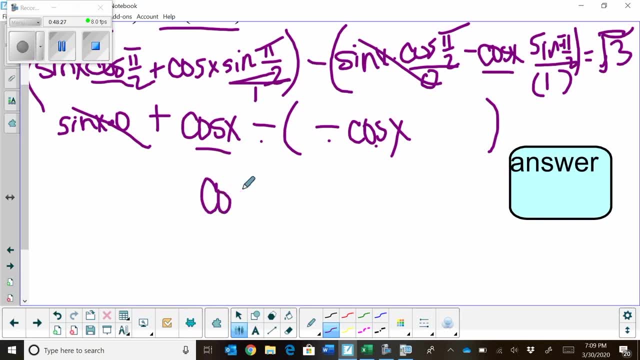 So what have we actually got left? We have cosine x minus a negative cosine x. Well, that double negative is just a positive, So that's going to be cosine x plus cosine x, And let's bring down our radical three.